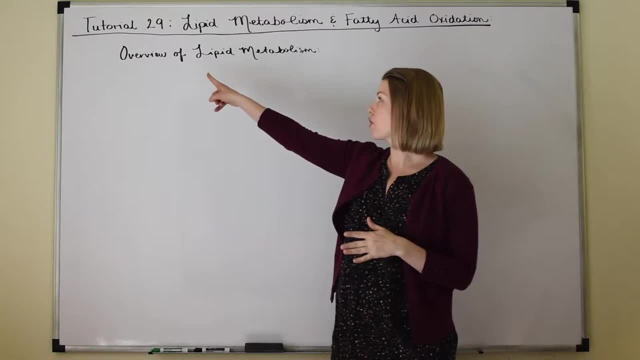 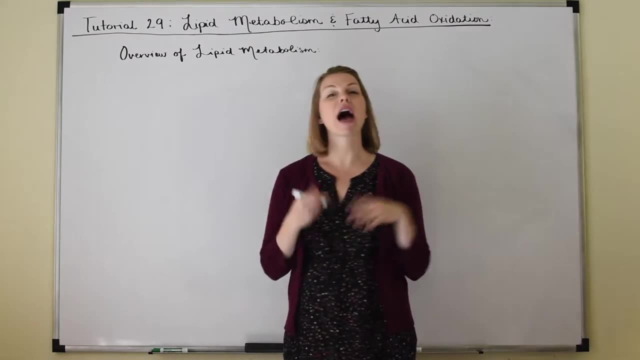 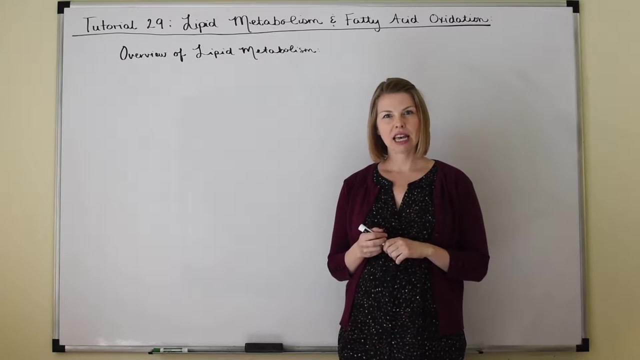 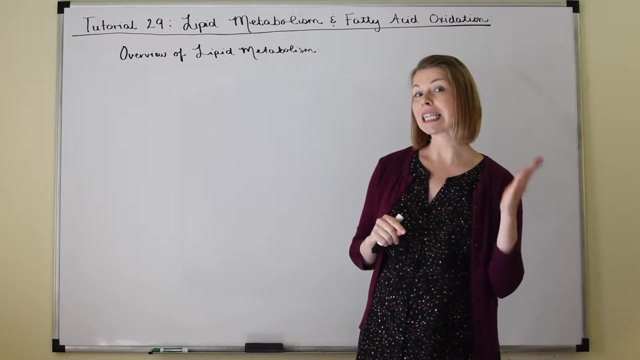 let's get started first with an overview of lipid metabolism. So we already know that the fats from our diet are primarily triglycerides, And during the digestion process the ester linkages within those triglycerides are hydrolyzed to free up glycerol and three fatty acids that can enter the 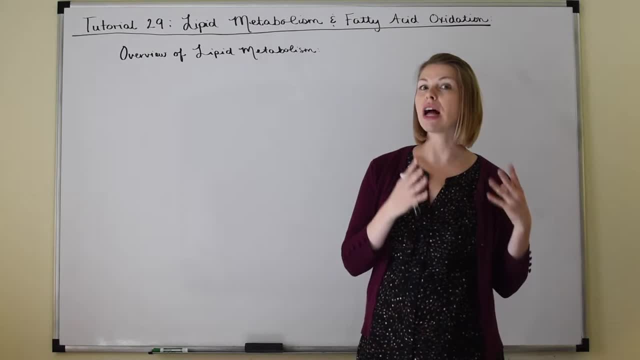 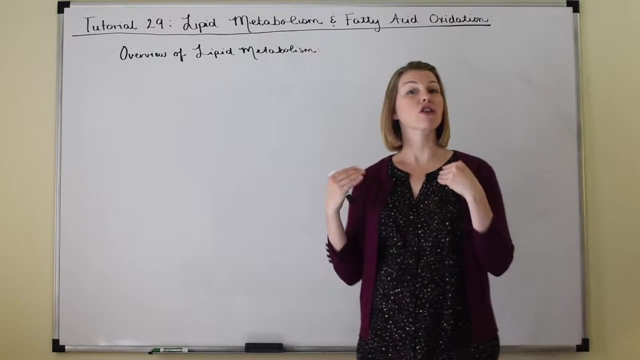 bloodstream. Those that are water soluble, like glycerol and the smaller fatty acids, can enter directly. Those that are longer chain, more hydrocarbon-like, that are not water soluble, are packaged into lipoproteins, So we talked about that. 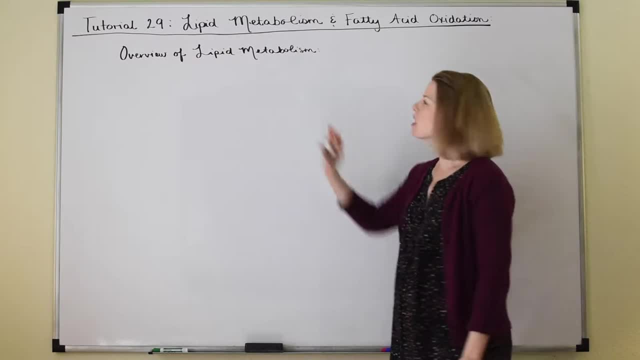 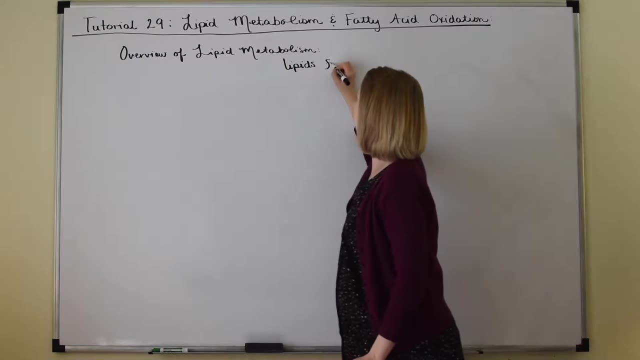 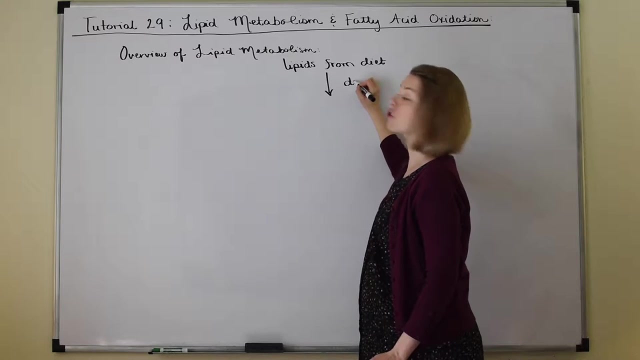 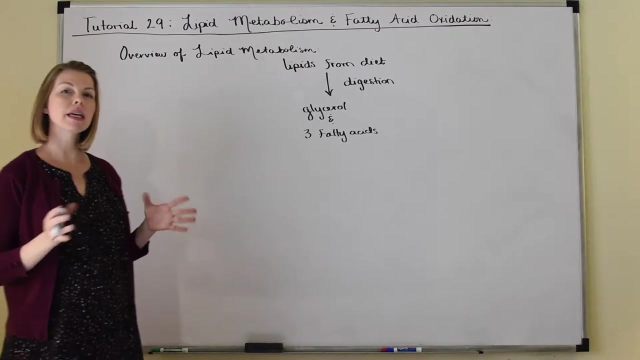 back in tutorial 27.. So let's just do a quick little note here. So lipids from our diet are hydrolyzed in the process of digestion to free up glycerol and the three fatty acids. Alright now, glycerol being a much different molecule than the three fatty. 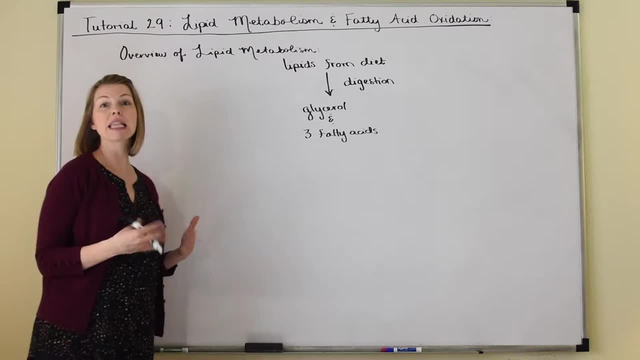 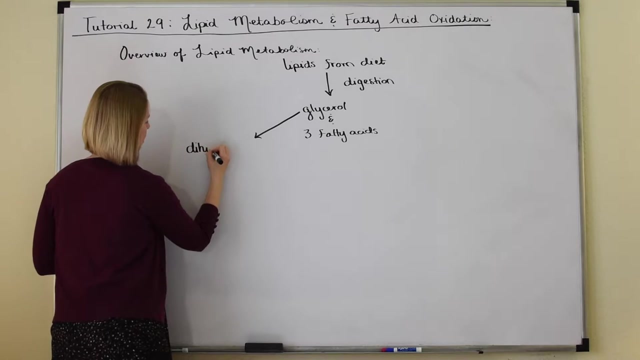 acids will undergo a different pathway in lipid metabolism. Glycerol can be converted into dihydroxyacetone phosphate, And you may recognize that name from the book The Lymph of the Lamp. The Lymph of the Lamp is a type of lymph that is caused by the use of lipid. 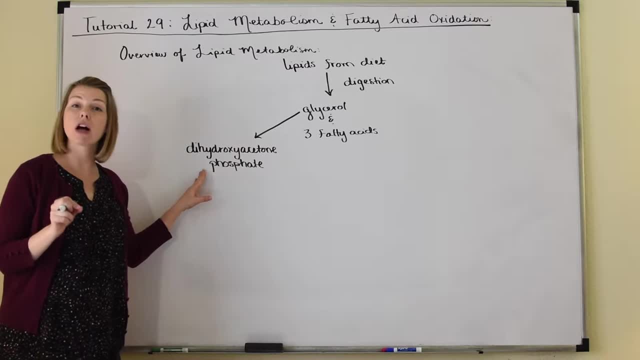 metabolism. Glycerol is also a type of lipid metabolism. Glycerol is a type of lipid metabolism from the process of glycolysis that we talked about in our last tutorial, tutorial 28.. Dihydroxyacetone is one of the three carbon products from step four of the glycolysis pathway. 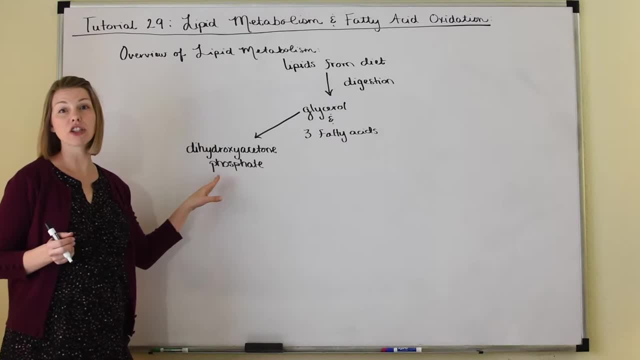 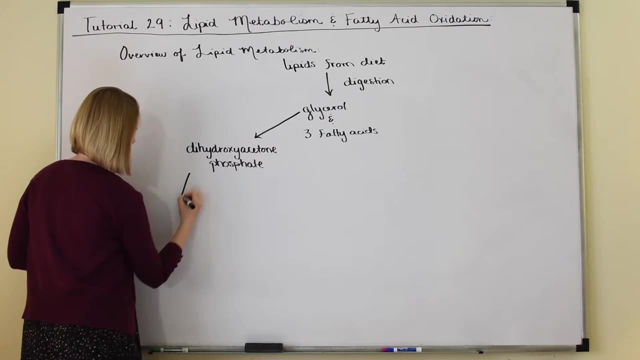 So that means that glycerol can enter the glycolysis pathway directly. So right here, which is the glycolysis pathway, where it can be converted into pyruvate, And we know then that pyruvate can be oxidized into acetyl coenzyme A. Through pyruvate, Pyruvate oxidation, And we know that acetyl coenzyme A can enter into the Krebs cycle- Be converted. the carbons from the foods that we eat are ultimately converted into carbon dioxide in that process. 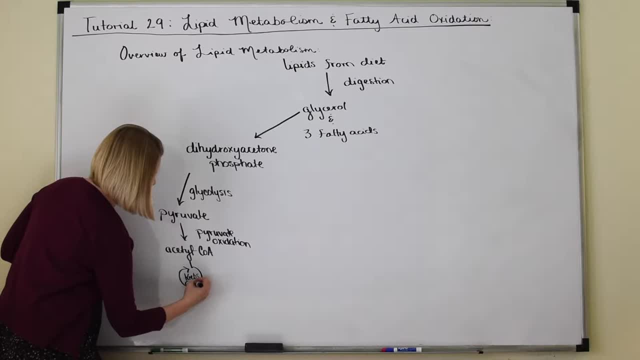 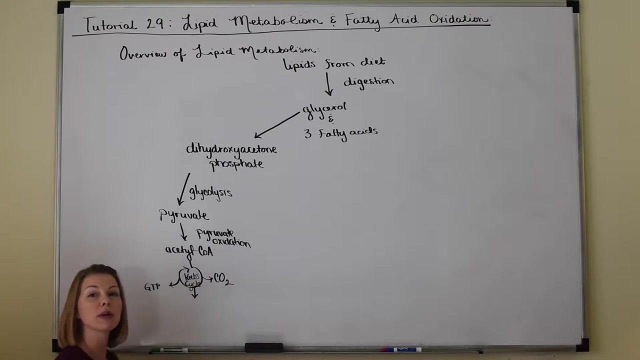 So right, Krebs cycle here, Fully oxidizing those carbons into carbon dioxide, Creating the high-energy molecule GTP. And because we have oxidation, coenzymes get reduced: Three coenzymes of NADH And one FADH2.. 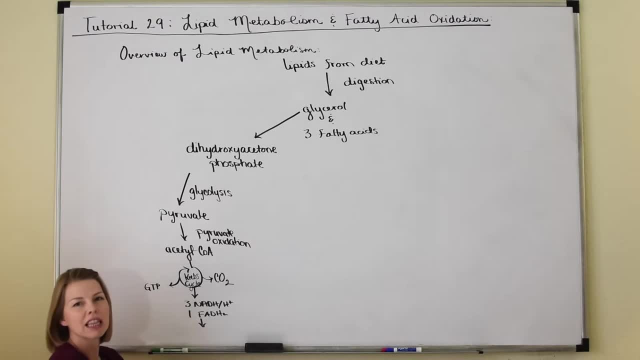 And we know that those coenzymes then get reoxidized in the electron transport chain. I'll show you ETC Giving us the reoxidized coenzymes: three NAD pluses and one FAD. And remember that the ultimate acceptor of the electrons and hydrogen ions in the electron transport chain 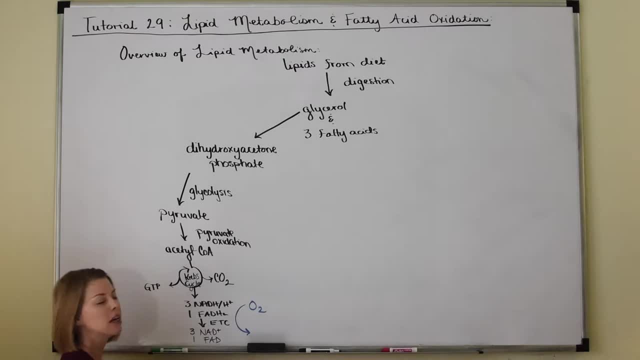 is oxygen from the air that we breathe which gets converted into water, H2O, And it's the energy from that highly exercised, It's our organic process that is harnessed to power. oxidative phosphorylation, That is, the phosphorylation of ADP into ATP. 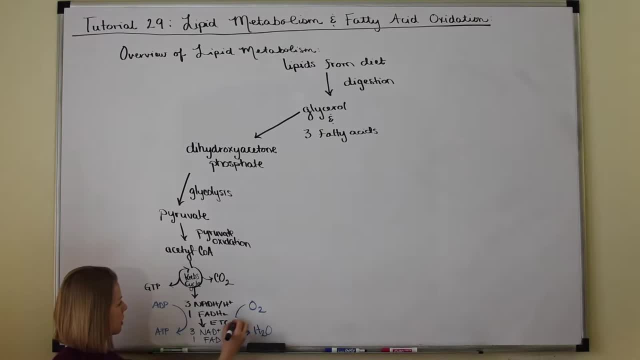 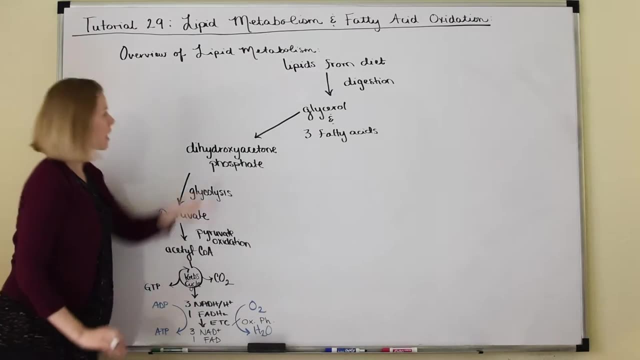 Okay, So all right here, Slash ox pho for oxidative phosphorylation. Okay, So that's one pathway for the glycerol to take. That glycerol is also- or excuse me That- dihyotroponics. 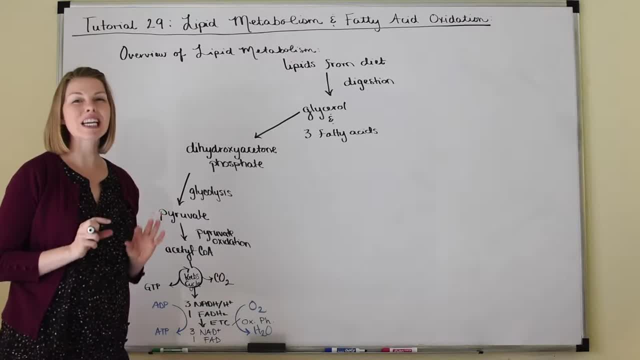 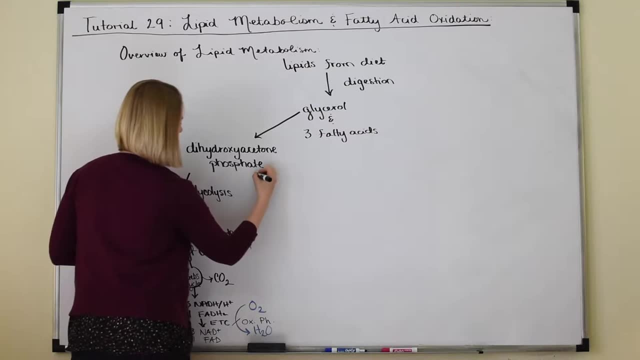 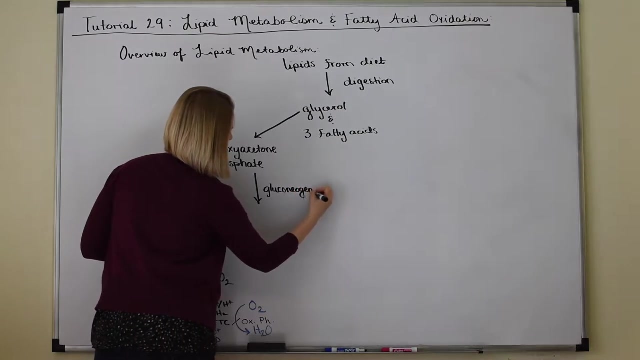 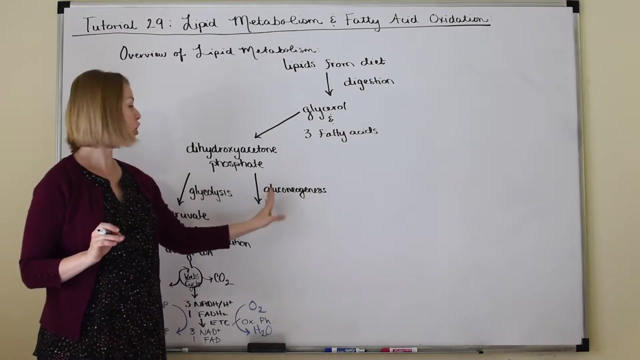 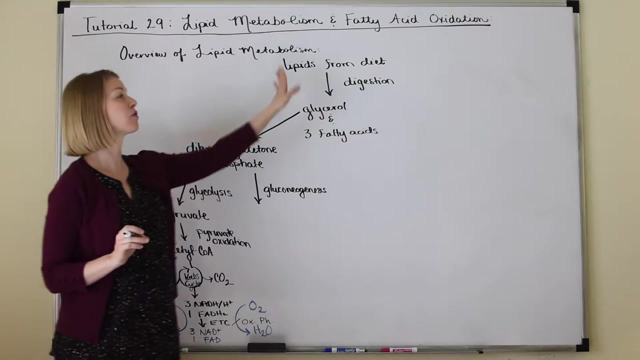 hydroxy acetone phosphate is also an intermediate in the pathway known as gluconeogenesis. So I'm going to write here gluconeogenesis, which is the synthesis genesis, the synthesis of glucose from non-carbohydrate sources. So this isn't coming from carbs, this is coming from lipids, in this case that dihydroxyacetone. 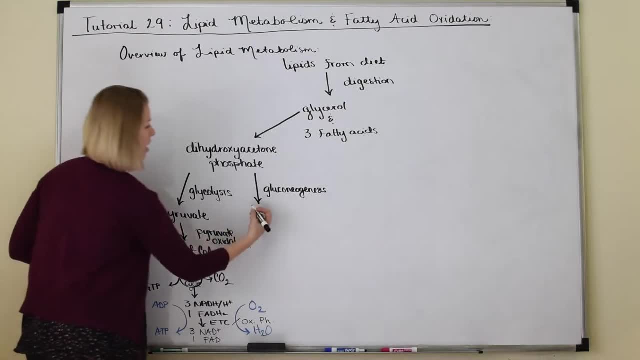 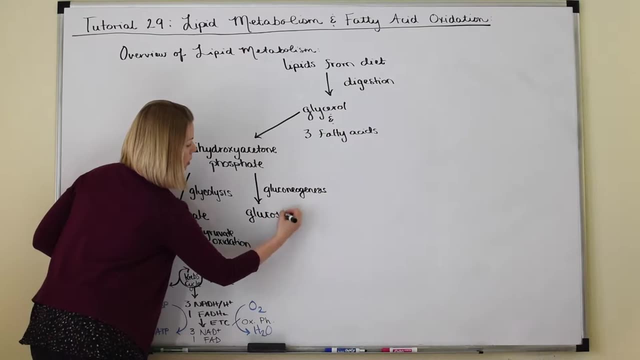 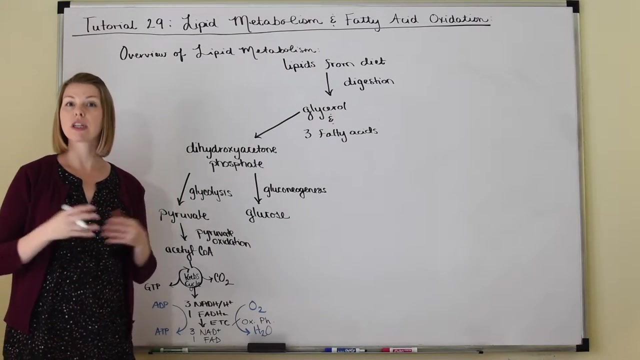 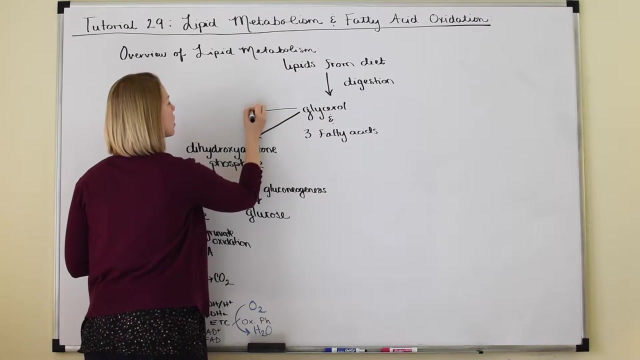 phosphate came from lipids in this case, and so that dihydroxyacetone phosphate from the glycerol can be used to synthesize glucose, which then can be further used in glycogenesis and stored as glycogen. Alright, last but not least, glycerol. 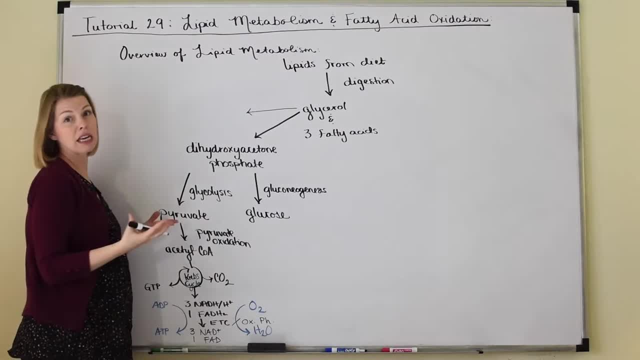 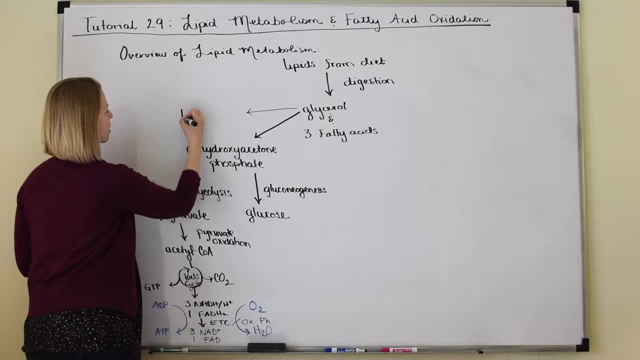 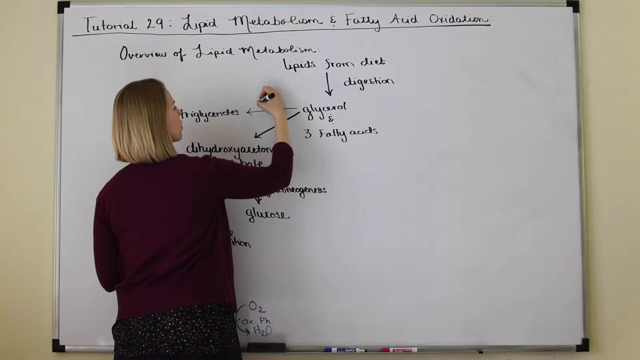 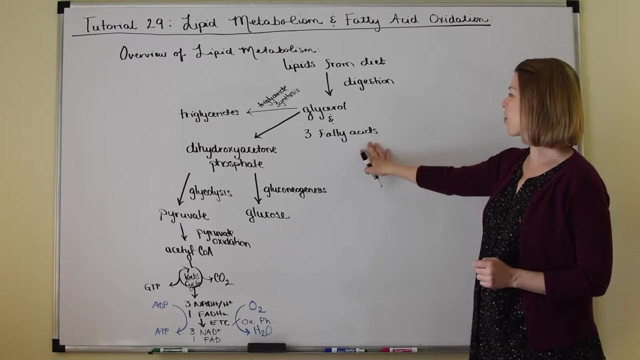 can also be used to re-synthesize triglycerides for storage in our cells. So that's right here, triglycerides, and we'll just call this triglyceride synthesis. Okay, so the many fates of glycerol. Alright, the three fatty acids will take a very different path. The three fatty 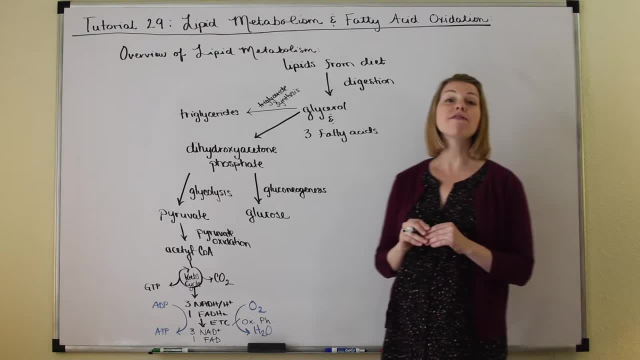 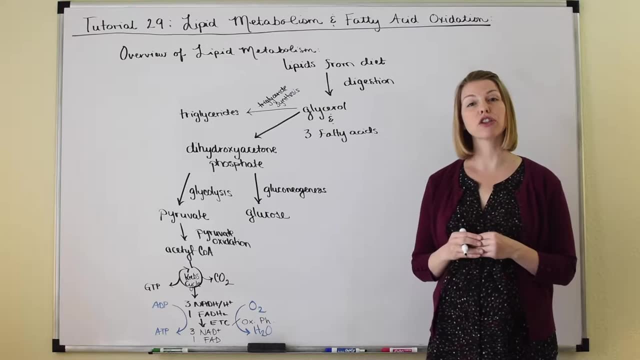 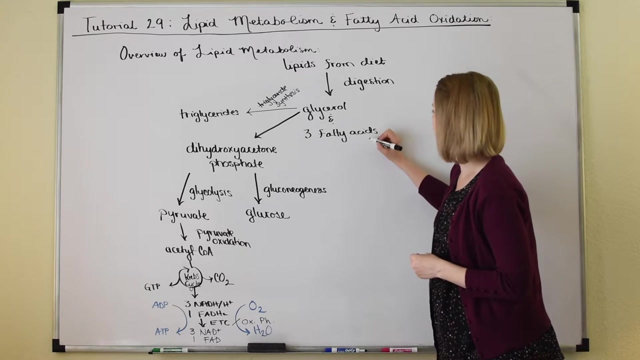 acids have to be oxidized via fatty acid oxidation in order to be converted into acetyl coenzyme A, which then can also enter the Krebs cycle, powering the electron transport chain and oxidative phosphorylation. So that's right here for our three fatty acids. they can be converted into acetyl coenzyme A, which can then be converted into acetyl coenzyme A. 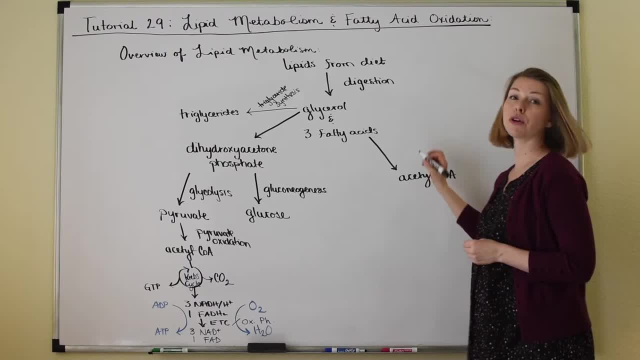 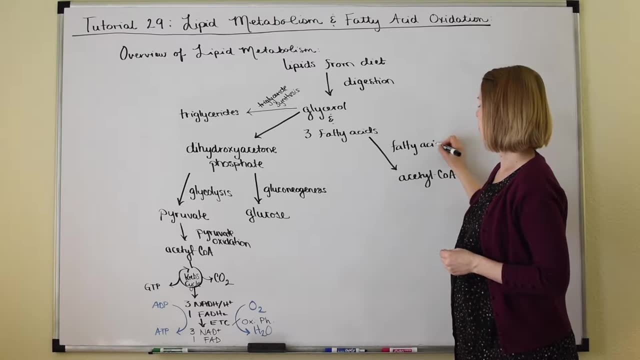 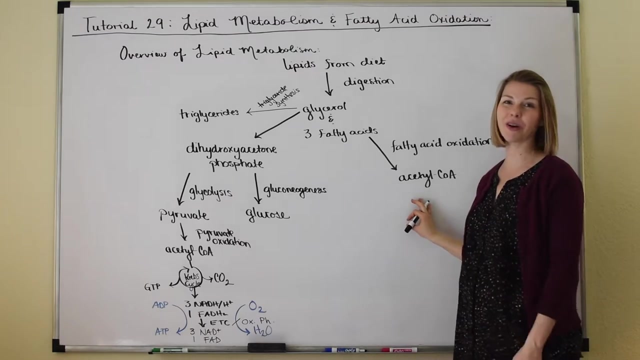 A through fatty acid oxidation. And then, of course, we know what can happen to acetyl coenzyme A. It does not matter whether it came from carbohydrates, fats or proteins in our diet. they can all be converted into acetyl coenzyme A. And once they're converted, 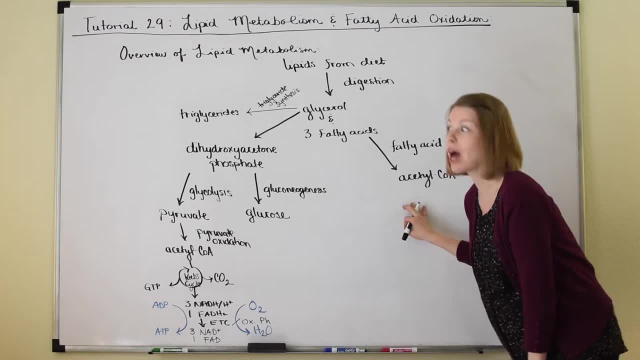 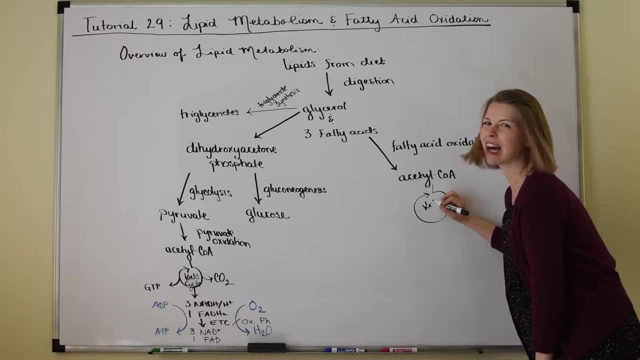 into acetyl coenzyme A. they can all enter into the Krebs cycle. I'm going to write that over here as well. It's a little redundant, but hopefully you're not too bored with that. Alright, we know that in the Krebs cycle the 2-carbon acetyl portion of acetyl coenzyme. 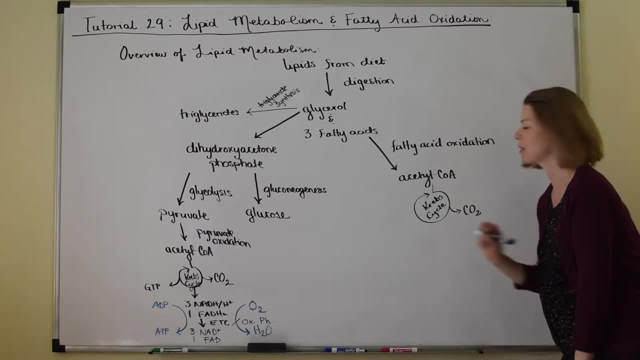 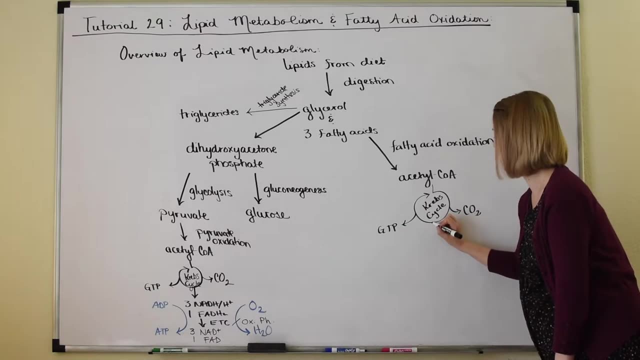 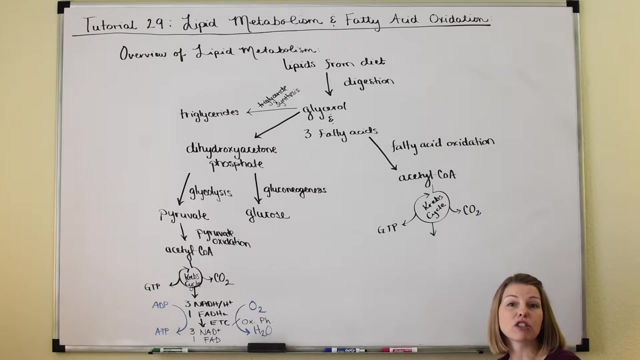 A gets converted to acetyl coenzyme. B converted, oxidized all the way into carbon dioxide. We get one high energy molecule of GTP for every turn we get in the Krebs cycle And, of course, oxidation is occurring. Every time we have an oxidation of a substrate, a coenzyme is going to be reduced. We get 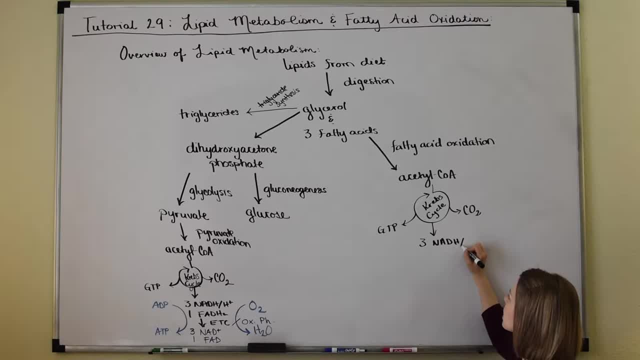 three reduced coenzymes of NADH and one of FADH2.. We know that those will be reoxidized in the electron transport chain. Ultimate acceptor of those electrons and hydrogen ions is oxygen from the air that we breathe to make H2O. 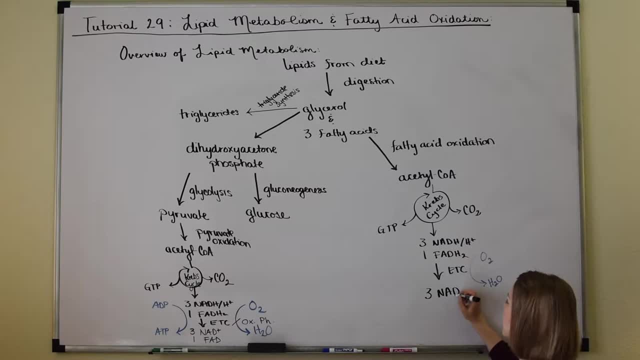 So we get three reoxidized coenzymes of NADH plus and one reoxidized FAD, And the energy released from the electron transport chain is harnessed and used to power oxidative phosphorylation, That is, the phosphorylation of ADP into ATP. So I'll just right here. 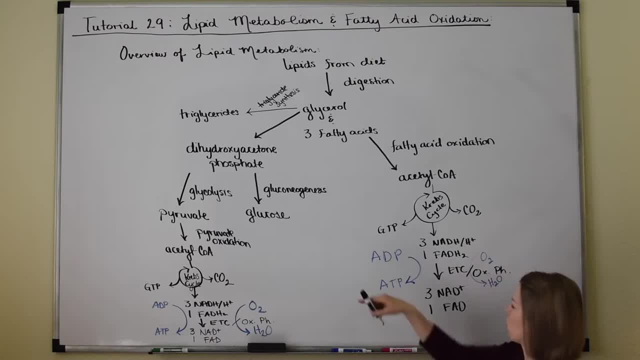 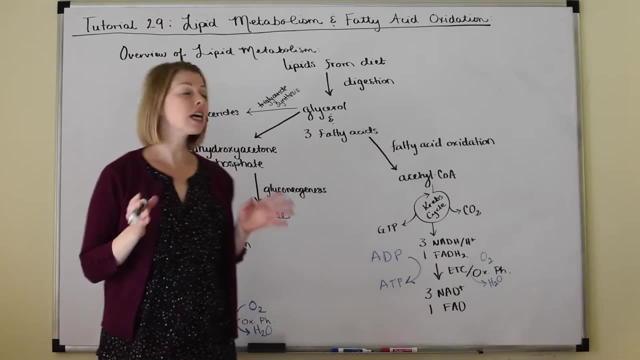 slash B-A-T-P. So we get three reoxidized coenzymes of NADH plus and one reoxidized FAD, And the energy released from the electron transport chain is harnessed and used to power oxidative ox foot, just like I did over there all right now. if the acetyl coenzyme a is in, 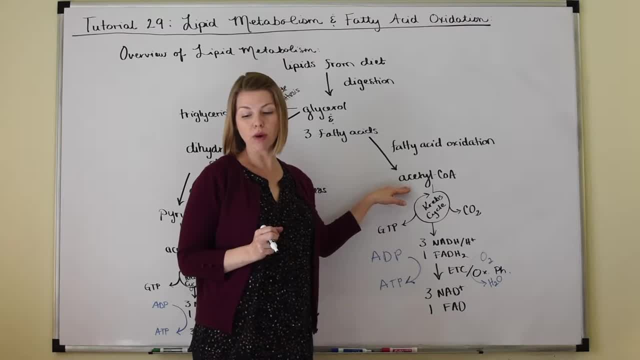 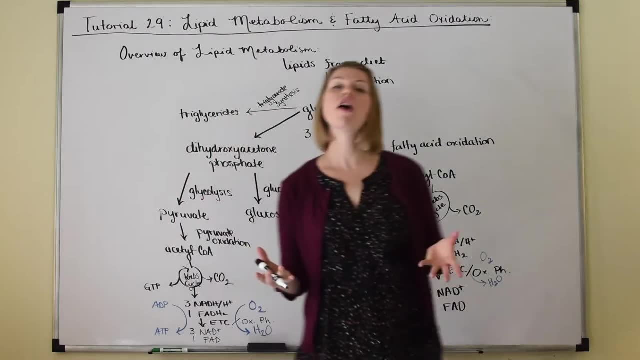 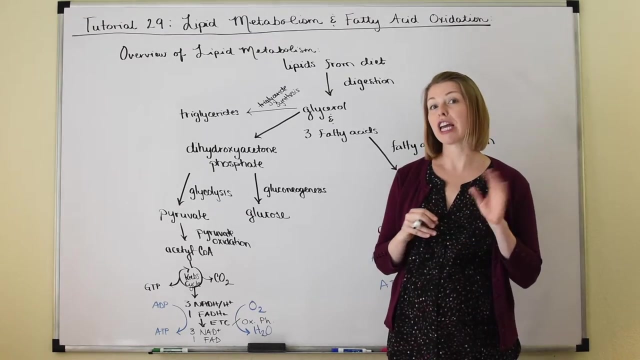 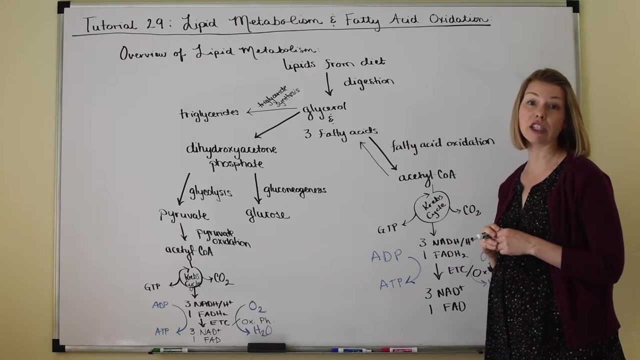 excessive amounts. we know already that excess acetyl coenzyme a can be used to synthesize fatty acids, which can then be used to synthesize triglycerides, which are stored for longer-term energy storage in our cells, and we learned that that process, the conversion of acetyl coenzyme a into fatty acids, is known as. 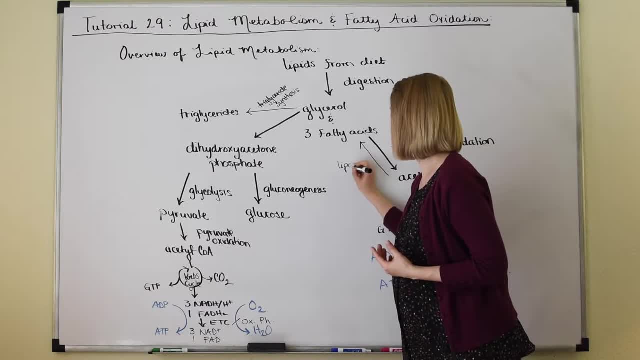 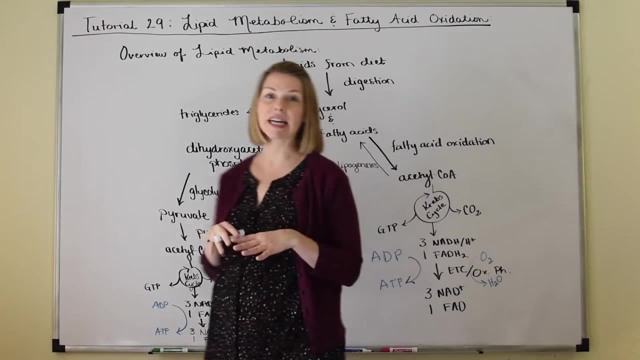 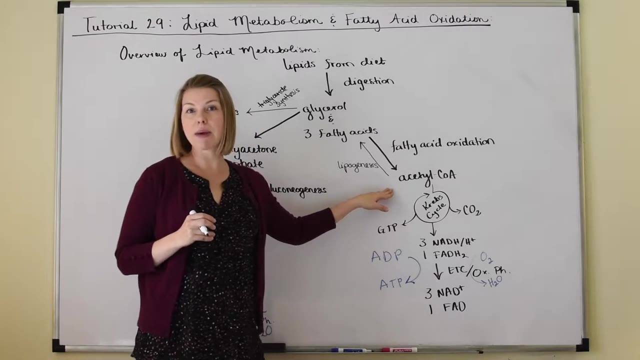 lipogenesis. so I'm gonna write that here, so that acetyl coenzyme a can be used to recreate fatty acids, which can then be used to recreate triglycerides for storage. but another fate of acetyl coenzyme a from the process of synthesizing fatty acids is that the 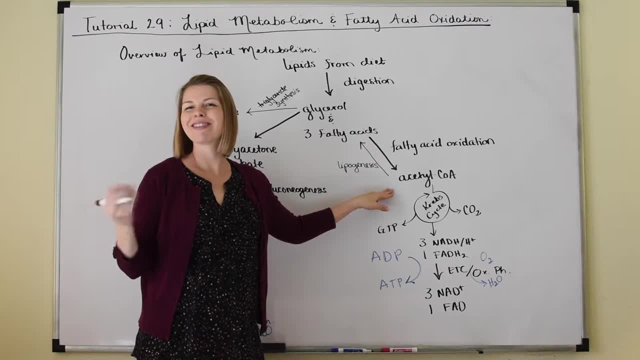 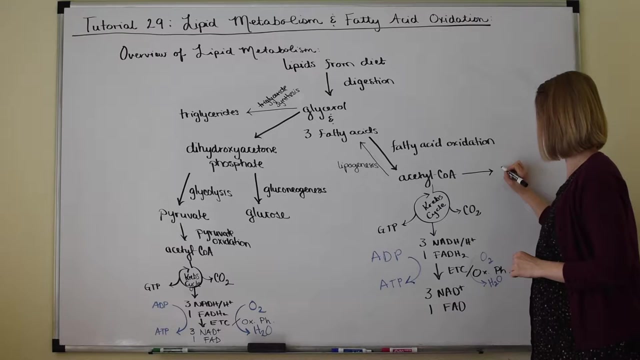 fatty acids that we eat, or fat stored and mobilized from our cells is conversion into a temporary energy storage called ketone bodies- so I'm gonna write that over here as well- and this is via a process known as ketogenesis, so the synthesis of ketone bodies, ketogenesis, and this happens primarily. 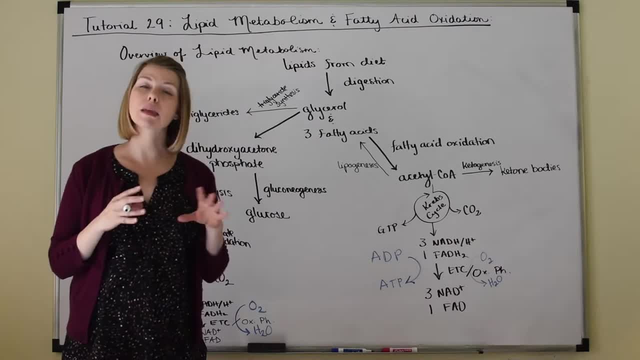 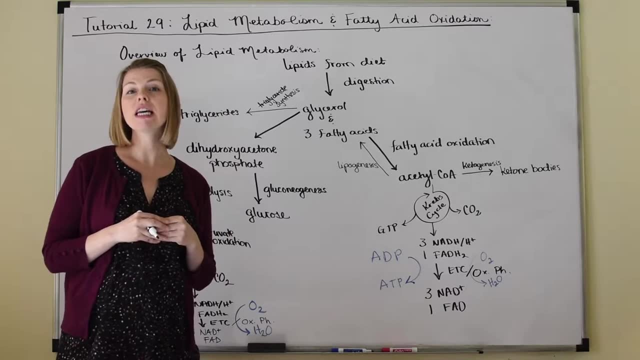 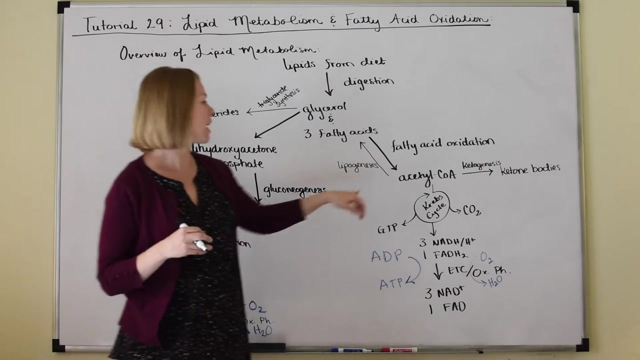 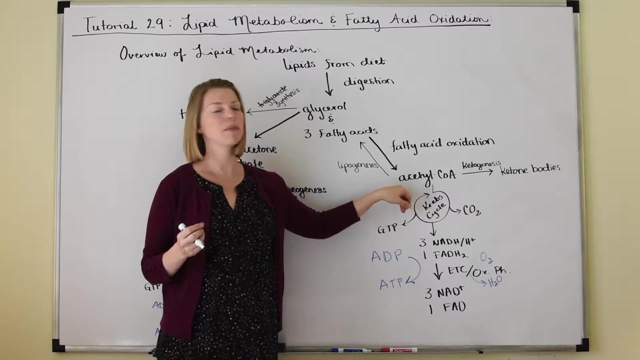 when glucose is in short supply and that means that fatty acid, fat mobilization is at a max. so fats are being mobilized from our fat cells and used to create acetyl coenzyme a. if there's too much acetyl coenzyme a, which will happen under these conditions, because some of the Krebs cycle. 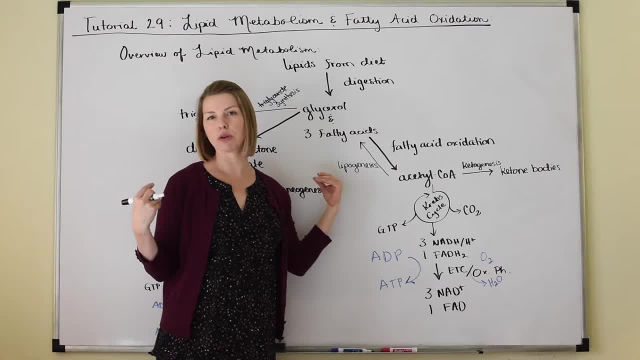 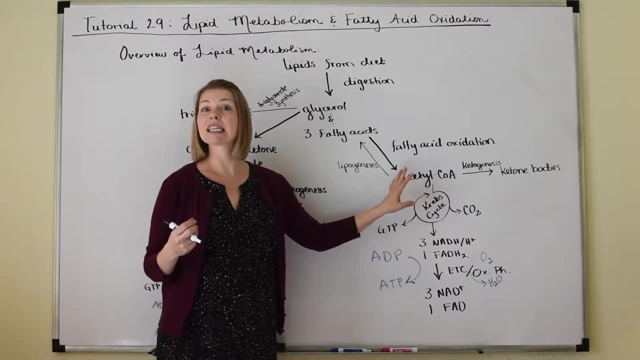 intermediates are actually used for the synthesis of glucose, then what we get is a slowdown of the Krebs cycle, a slow down in the uptake of the Sal化 Acetyl Coenzyme EA, and excess acetyl coenzyme a can be stored in a temporary energy storage. 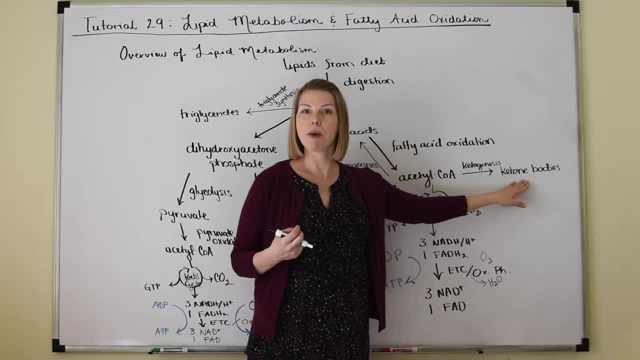 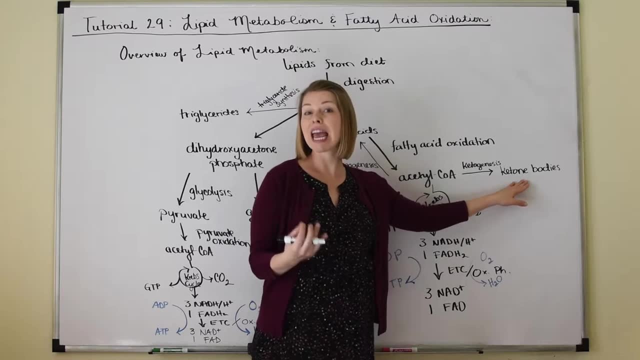 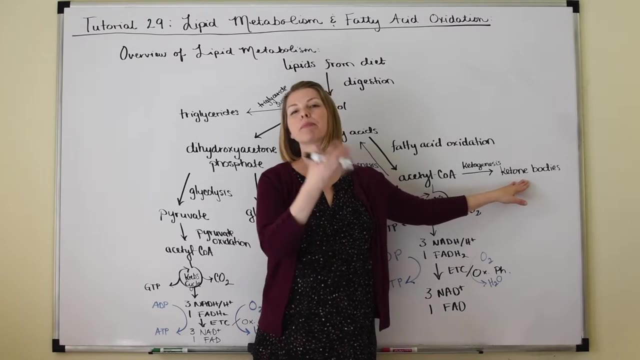 method of ketogenesis to make these ketone bodies- and these ketone bodies are very water soluble molecules, they can be absorbed directly into the bloodstream- and two cells that can then later catabolize the ketone bodies, returning them back into acetyl coenzyme A and passing them through the Krebs cycle, electron transport and an oxidative 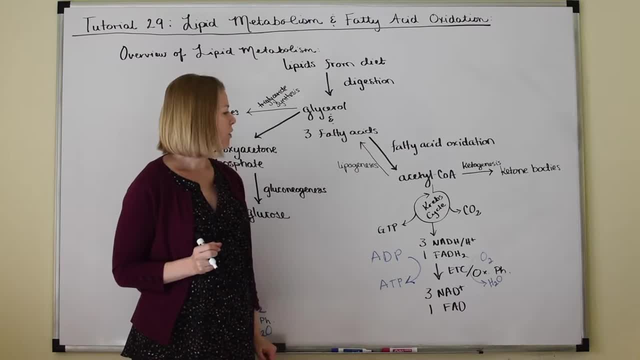 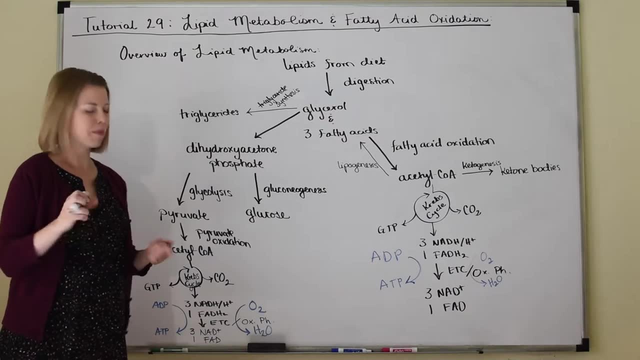 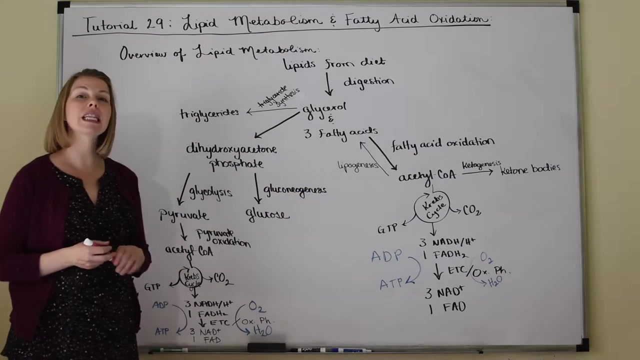 phosphorylation for energy needs. All right, so that's a pretty big overview of metabolism there. I know it looks a little complicated, but we're not going to focus on all of these aspects today. What we're focused on today is really the catabolic pathway for the three fatty acids. 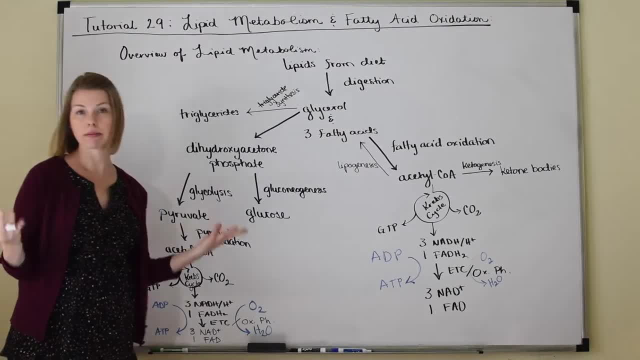 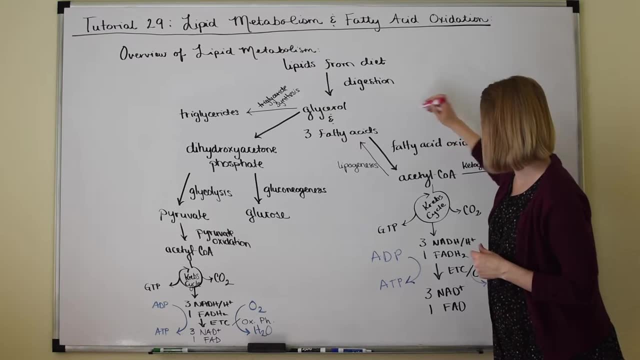 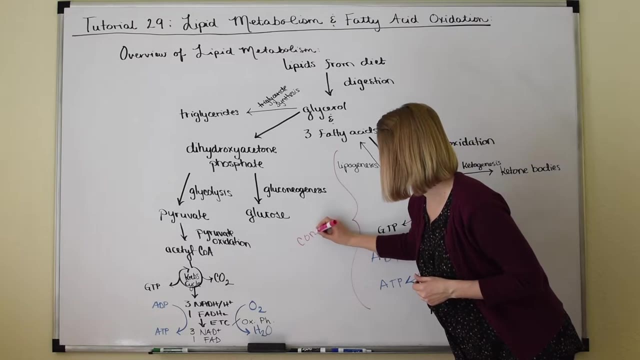 that are released from the foods that we eat, or the triglycerides that are mobilized from fat storage. So we're focused on this pathway. here Let's see The complete catabolism Of fatty acids. Okay, that's our focus for today. Now we already talked about the Krebs cycle. 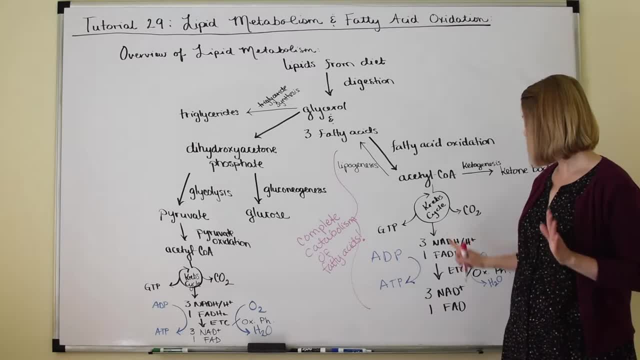 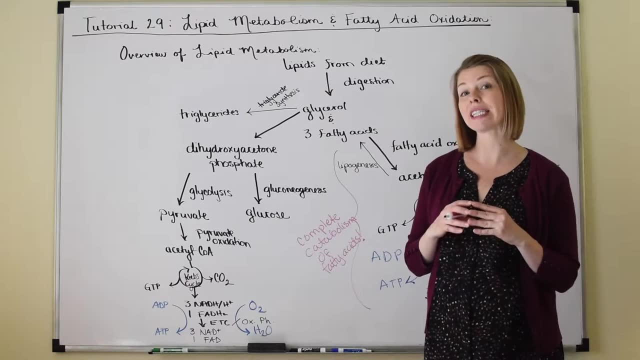 the eight steps of the Krebs cycle, as well as the electron transport chain and oxidative phosphorylation, in quite a bit of detail in tutorial 27.. So if you skip tutorial 27,, you're going to see that I've talked about the eight steps of the Krebs cycle. 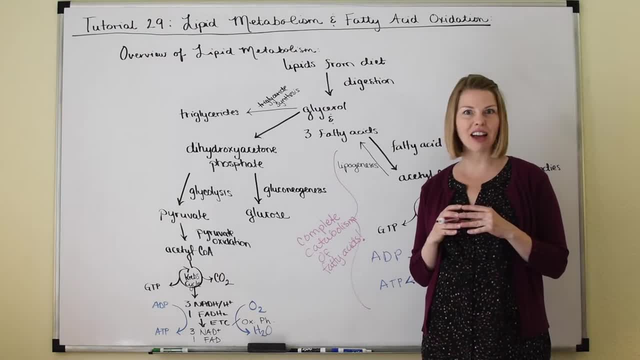 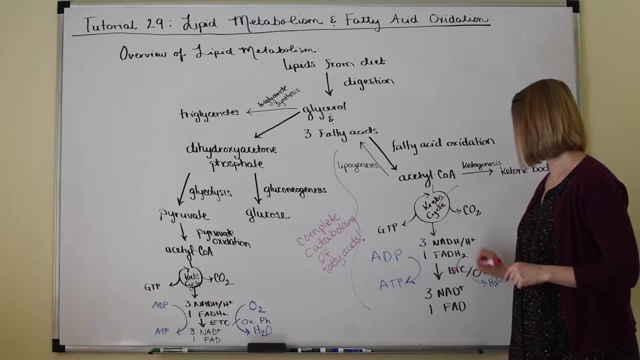 I highly recommend you go back and watch that tutorial video so that you know what's going on in the Krebs cycle, also known as the citric acid cycle, the electron transport chain and oxidative phosphorylation, because I'm not going to go into details on those catabolic processes. 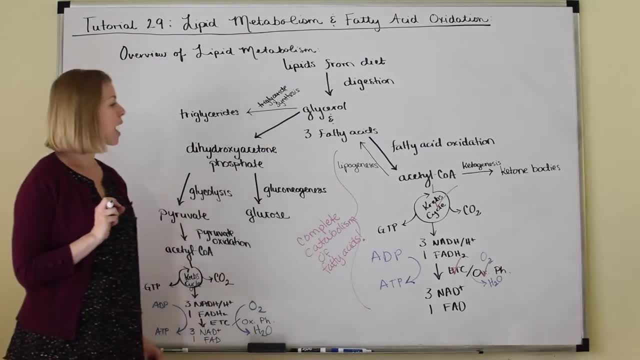 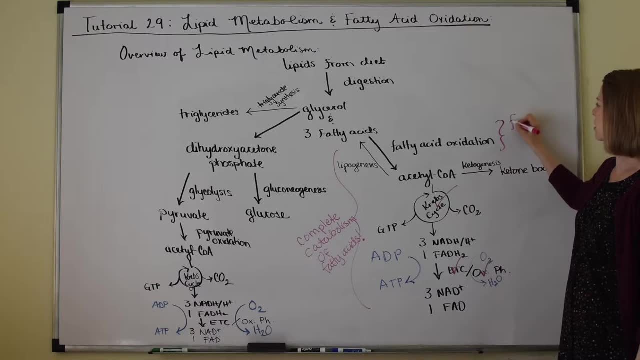 in this tutorial. We've already done that, So that means that all we really have to focus on for today is fatty acid oxidation. So, right here, this is the focus. So let's go ahead and erase all of this so that we can start talking in more details about fatty acid oxidation. 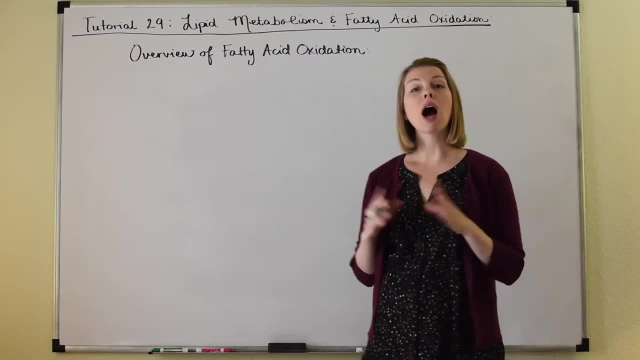 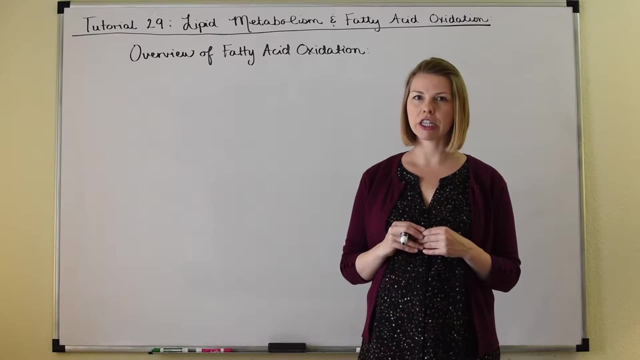 So I like to start out with an overview of these catabolic processes first. I think that's a lot easier than just throwing a bunch of reactions up on the board. I like to start out with an overview of these catabolic processes first. I think that's a lot easier than just throwing a bunch of reactions up on the board. 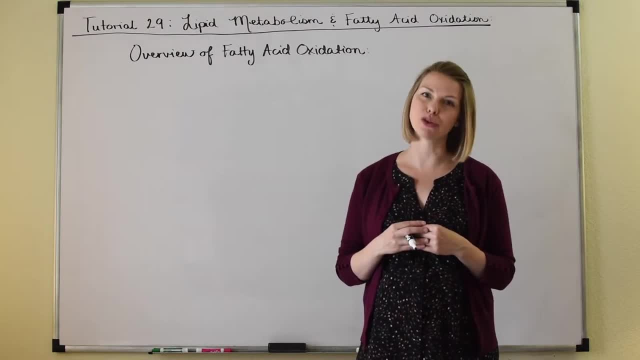 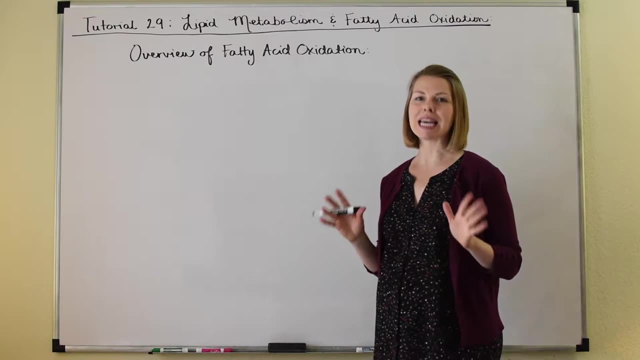 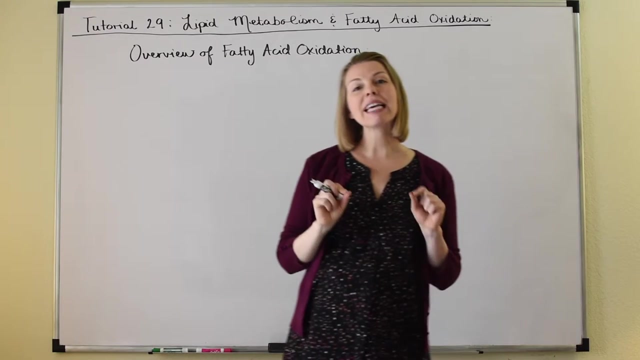 Which is kind of overwhelming for someone who is new to this information. So all we're doing right now is giving an overview of what is happening in the catabolic process known as fatty acid oxidation. Well, first of all, the fatty acid has to be activated. 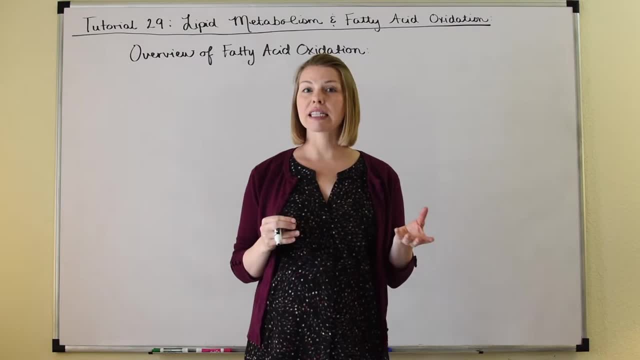 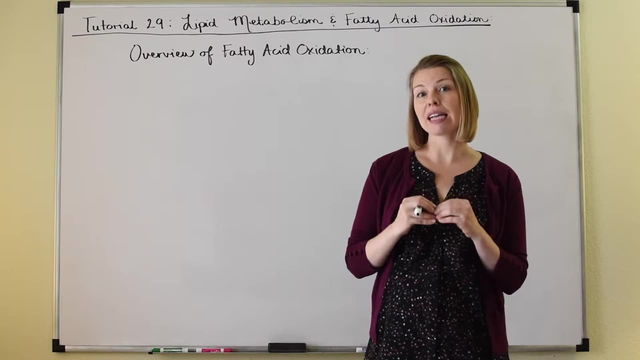 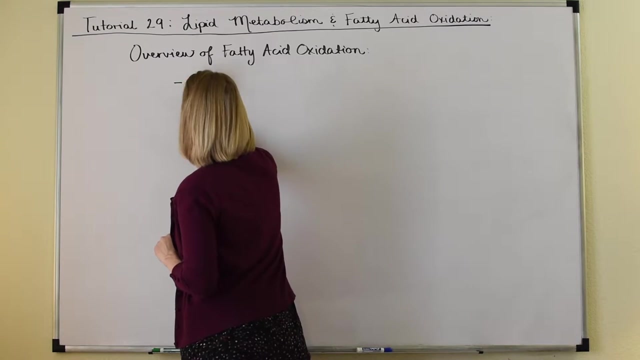 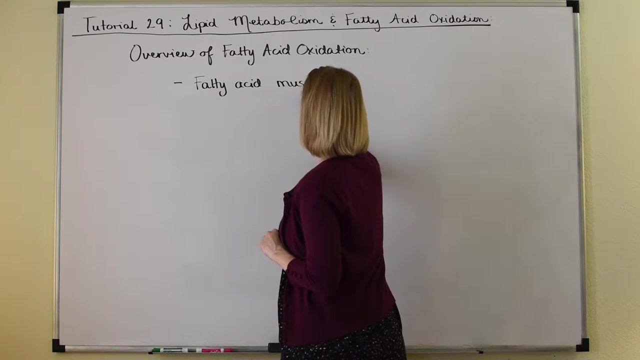 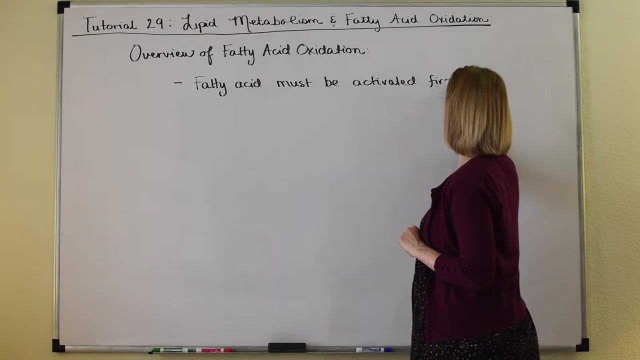 And all that means is that the fatty acid is going to be combined with a coenzyme A molecule And making up a molecule name Known as a fatty acyl coenzyme A. So let's write that up on the board. The fatty acid must be activated first. 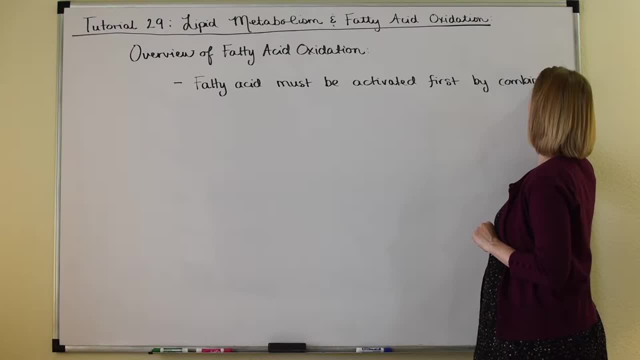 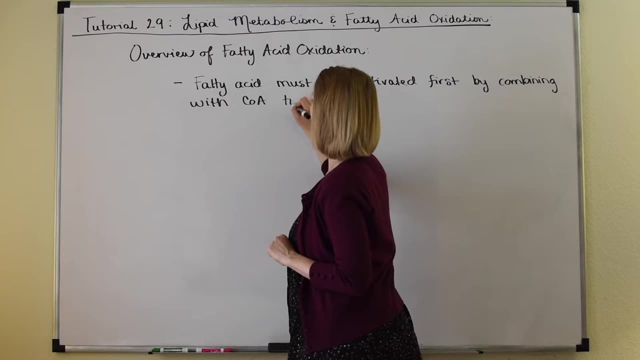 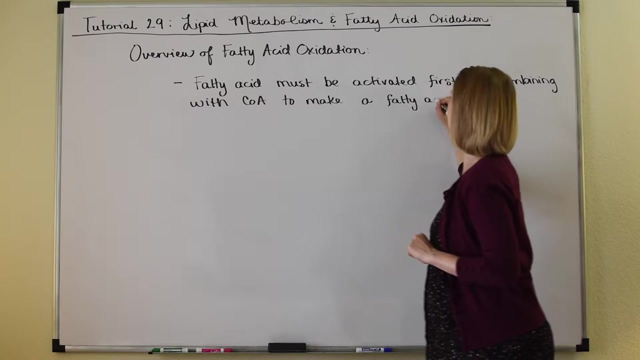 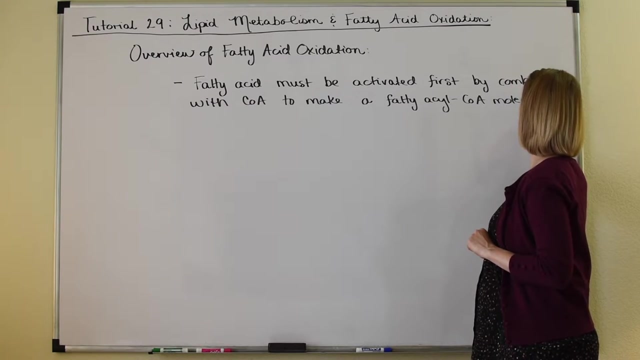 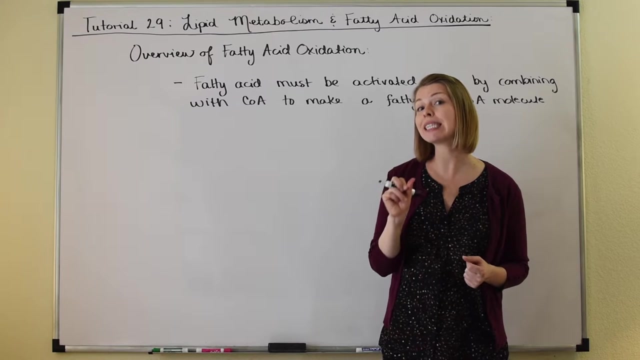 By combining With Coenzyme A To make A fatty acyl coenzyme, A molecule, And this process occurs within the cytosol of the cell And it requires 2 ATP to activate a fatty acid. So let's write that down as well. Occurs within the cytosol And I'm going to write: minus 2 ATP Takes 2 ATP to activate a fatty acid For fatty acid oxidation. Okay, Now that the fatty acid has been activated, Converted into a fatty acyl coenzyme, A molecule 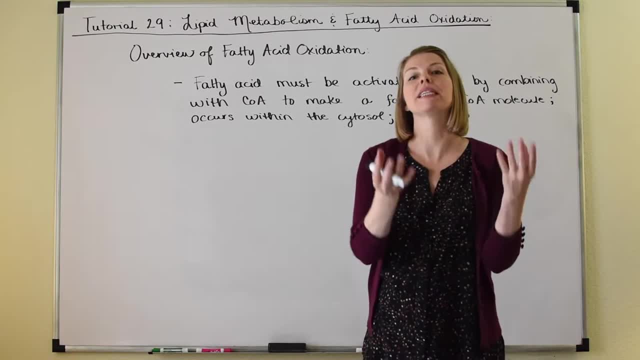 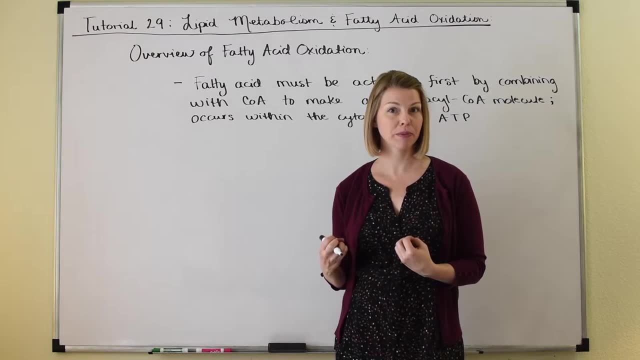 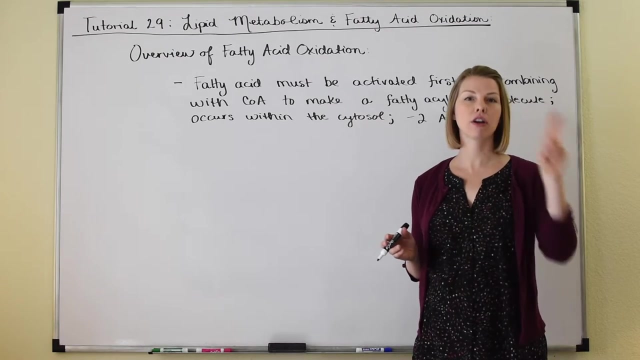 That fatty acyl coenzyme A molecule can be taken into the mitochondrial matrix And that is where the fatty acid oxidation will occur. And all that happens in that process Is that 2 carbons are cleaved off at a time As acetyl coenzyme A. 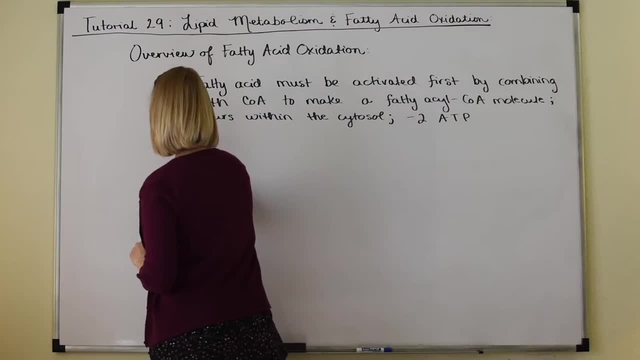 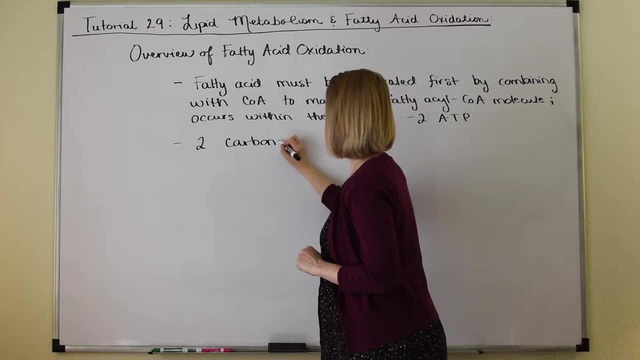 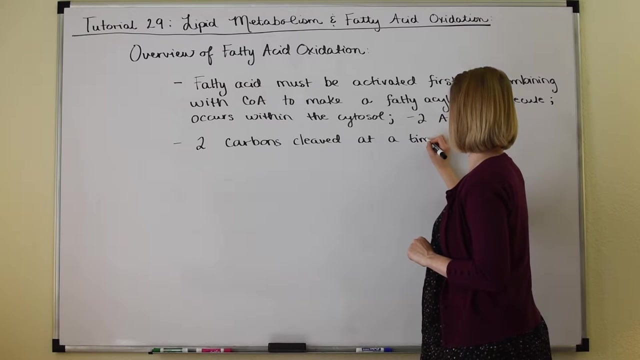 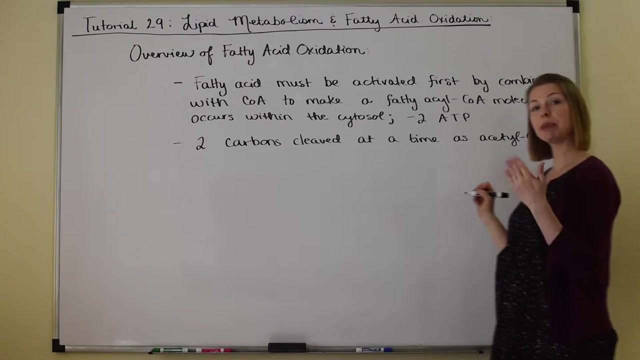 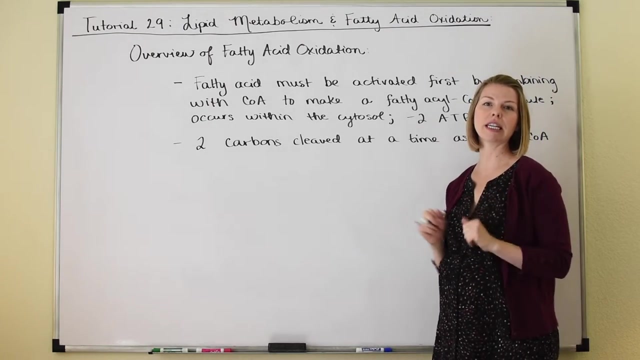 So let's write that up here: 2 carbons cleaved at a time As acetyl coenzyme A, And this will happen until all the carbons in the chain From the fatty acid chain Are converted into acetyl coenzyme A. 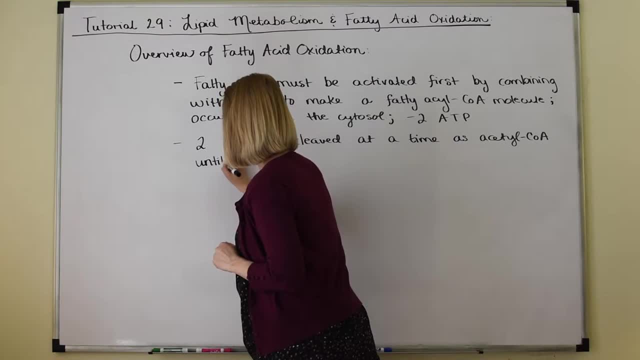 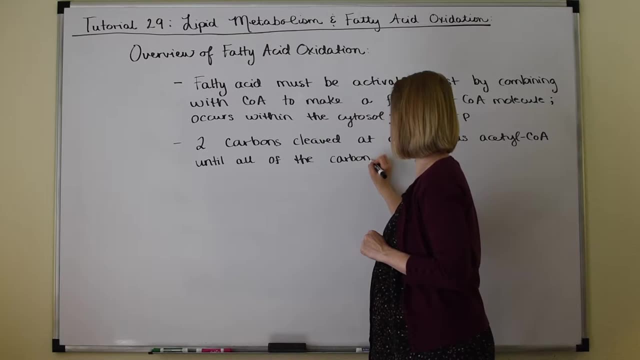 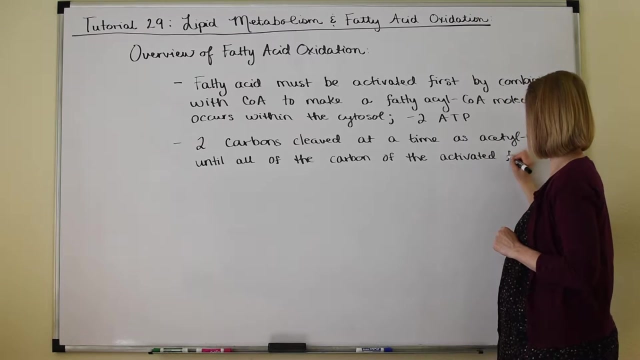 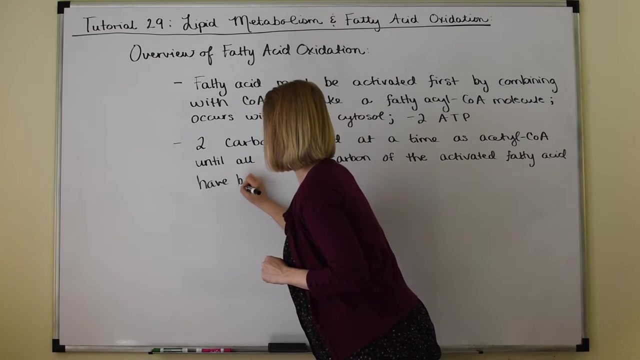 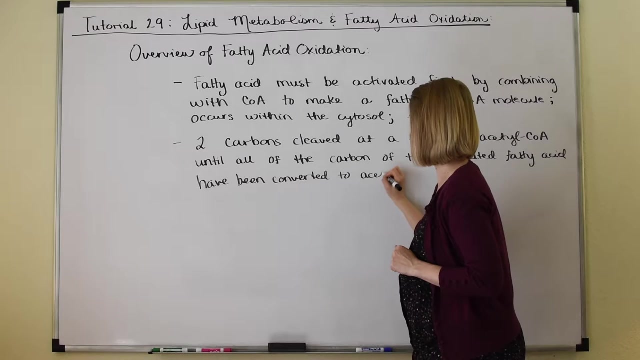 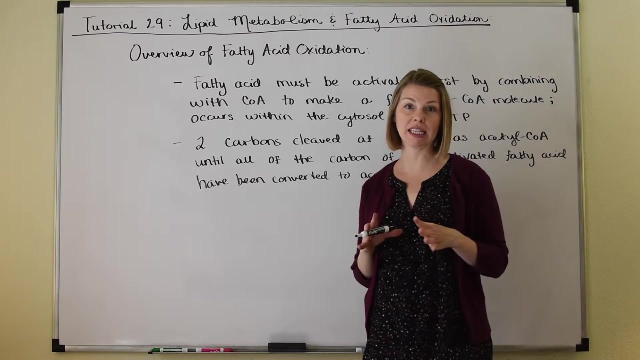 So I'm going to write here Until all of the carbon Of the activated fatty acid Have been converted, Converted To Acetyl coenzyme A. Now notice that this process Is a spiral, Not a cycle. Okay, The Krebs cycle. 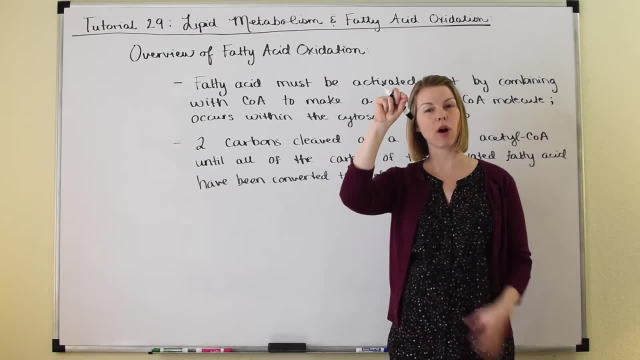 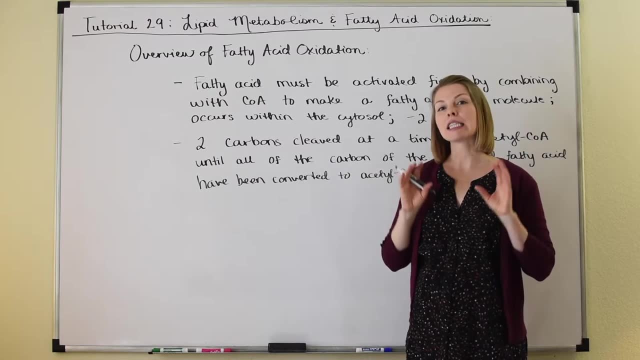 Is a cycle. It's a cycle because The reactor from step 1 is a product from step 8.. And it just keeps going and going and feeding itself In each turn. A spiral is different, Because in a spiral This is just going to continue to occur. 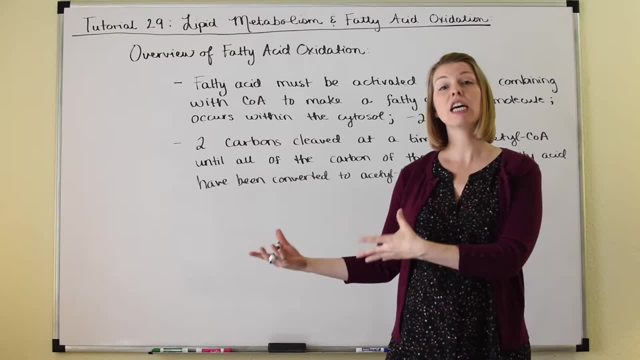 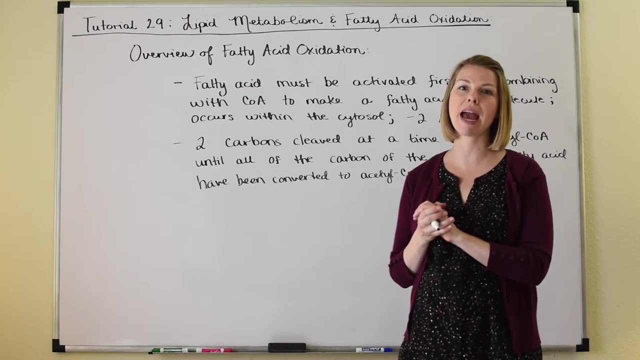 Until all the carbons of the fat Activated fatty acid Are gone, And then It terminates. It ends. All the carbons have been converted into acetyl coenzyme A, So let's write that down as well, That this 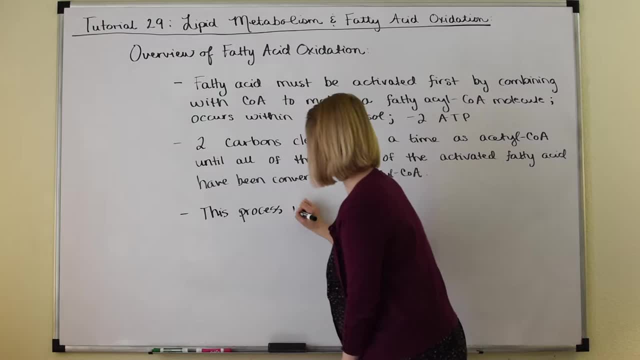 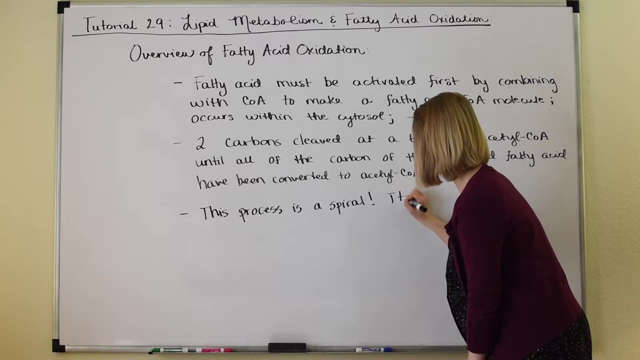 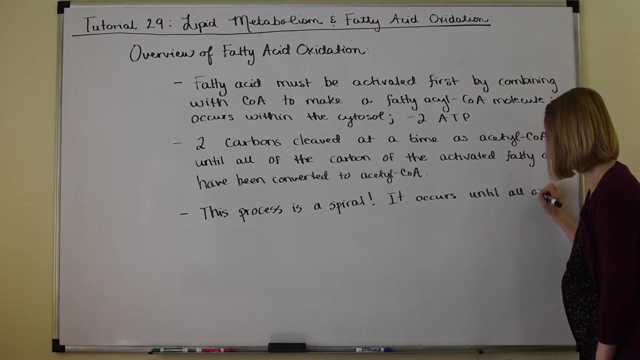 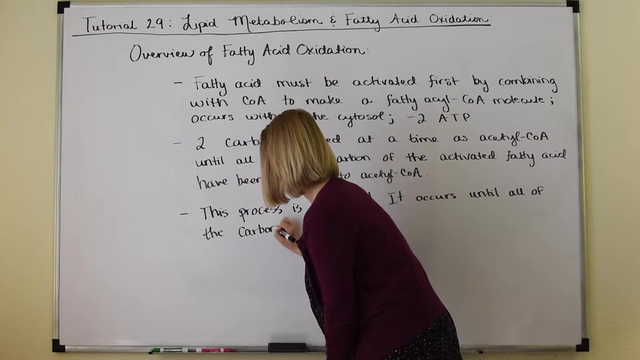 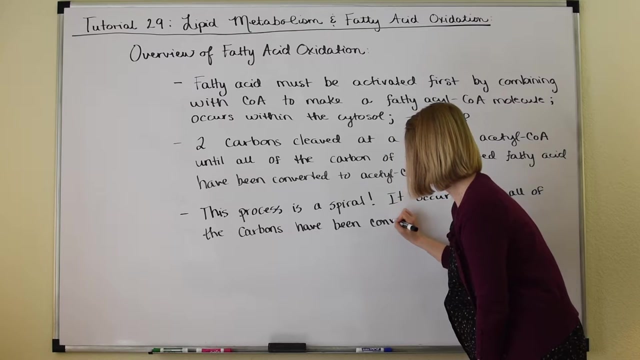 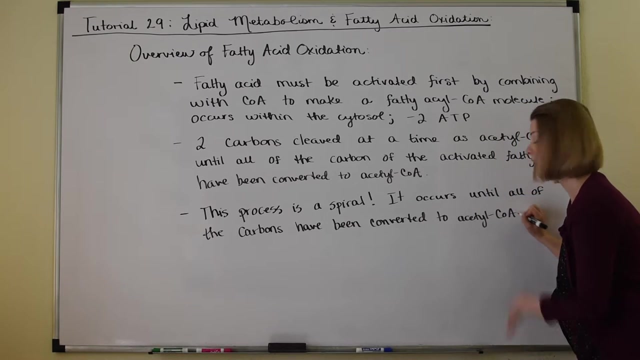 Process Is A spiral Meaning. It occurs Until All Of The carbon Carbons Have Been Converted To Acetyl Coenzyme A, And then it's done. Okay, No more carbon to convert. 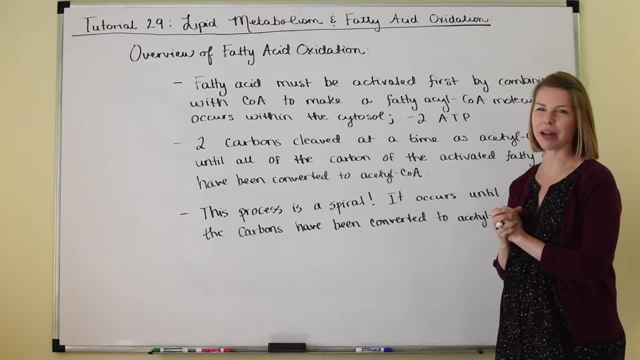 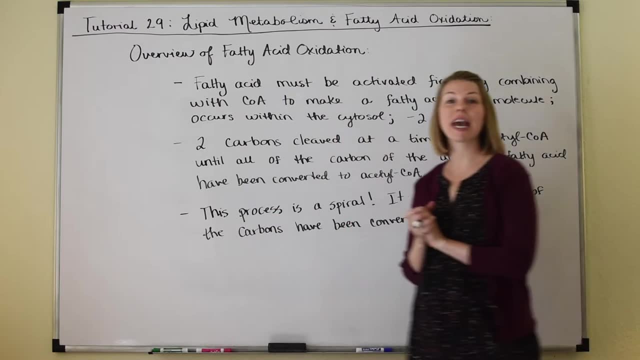 Into acetyl coenzyme A For that particular Activated fatty acid. Anyway, All right. So let's go ahead And zoom in now To slide number 3. So that we can look At these steps In more detail. 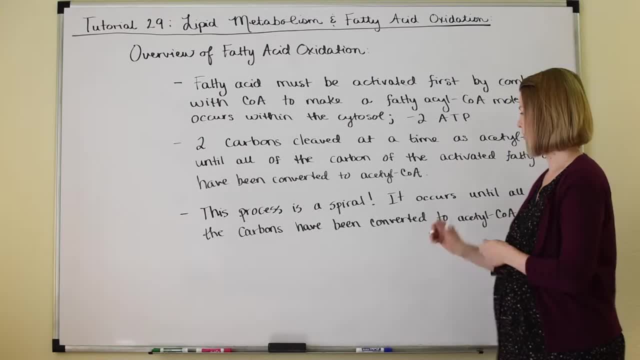 Okay, So here we are, Zoomed in to slide 3. And we're going to talk about the four steps Of the fatty acid spiral In detail. And here we are: We're going to talk about The four steps. 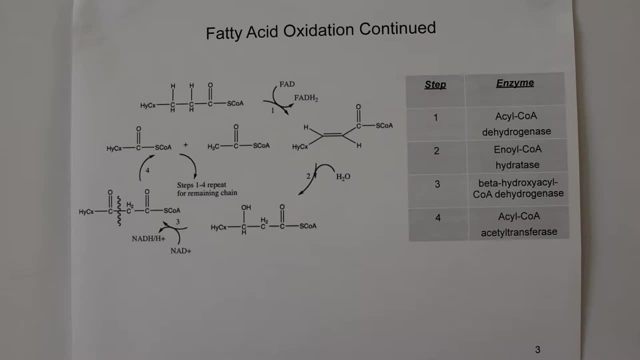 Of the fatty acid spiral In detail. And here we are. We're going to talk about The four steps Of the fatty acid spiral And you can see Over here That we have our Activated Fatty acid. 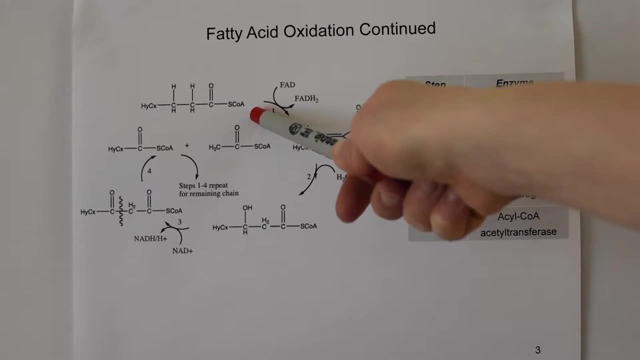 And remember That all That happens In fatty acid Activation Is that It's combined With the coenzyme A To make A molecule Known as a fatty Acyl Coenzyme A molecule, And that occurs. 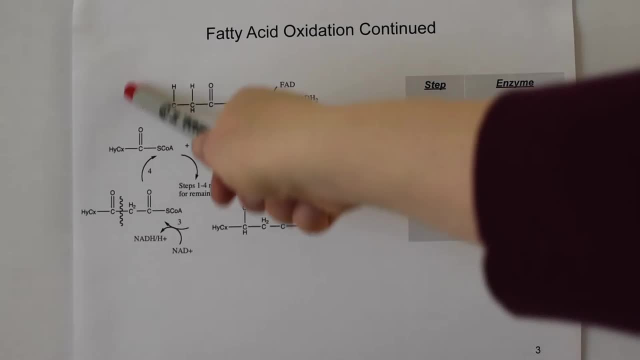 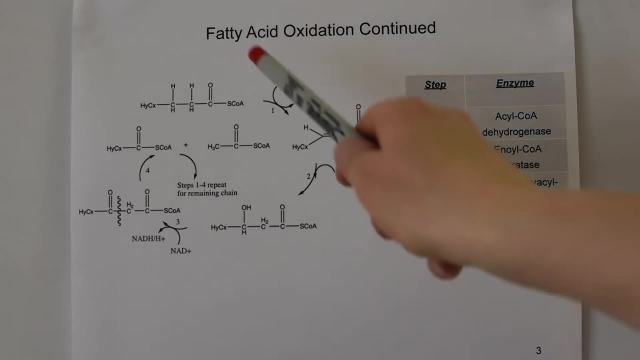 In the Cytosol Of the cell, And then the activated fatty acid, The fatty Acyl Coenzyme, Can be taken Into the mitochondrial matrix, And it's within the mitochondrial matrix That this spiral Will occur. 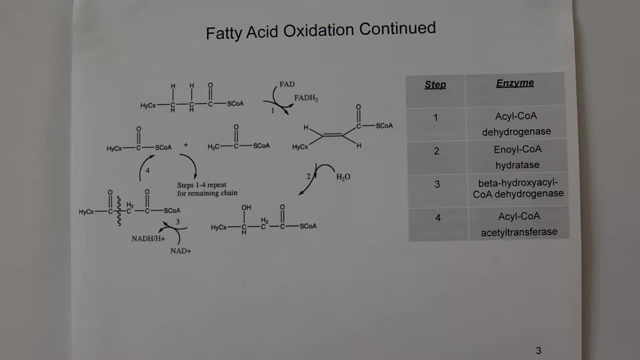 The four reactions Of the fatty acid spiral. All right, So on step one, That activated Fatty acid Is oxidized Through the removal Of two hydrogen To create This trans Double bond Between the alpha And the beta. 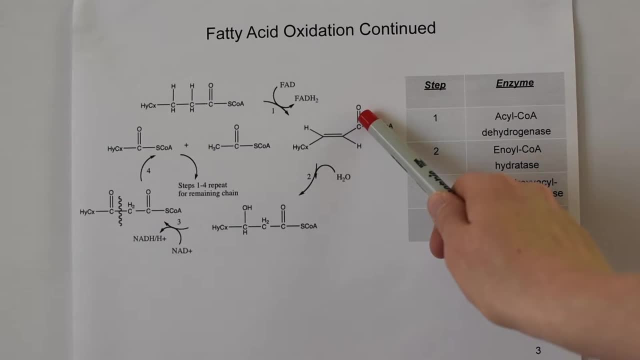 Carbon, Remember, The alpha Carbon Is One position From the carbonyl And the beta Is One position And the beta Is Two positions From the carbonyl K. Now, of course, Since our substrate's 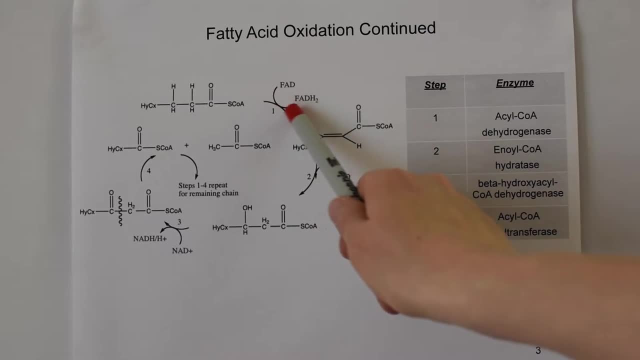 Being oxidized, We would expect A coenzyme To be reduced. That's exactly What we see here. The coenzyme Being reduced On step one Is FAD To FADH2.. That double bond Is then hydrated. 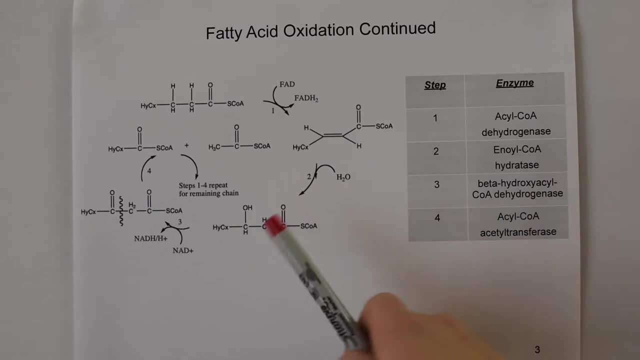 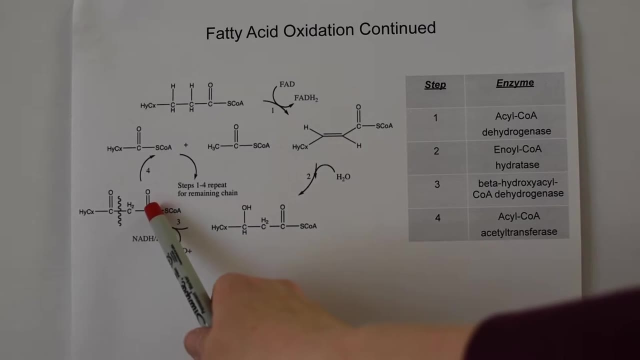 In step number two, Giving us An alcohol At the beta position Which is then Oxidized In step number two. Giving us An alcohol Which is then Oxidized In step three To a ketone. 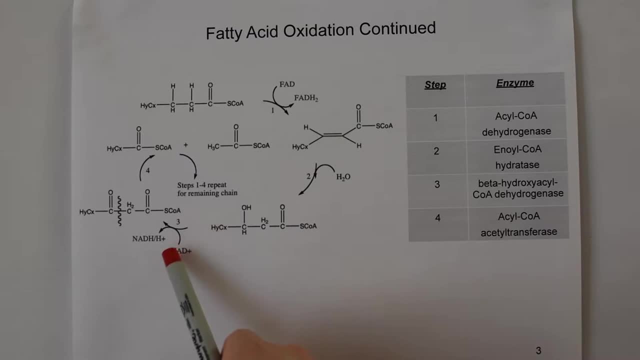 Since The substrate's Being oxidized In step three, A coenzyme Has to be reduced. In step three, The coenzyme Is NAD+, Being reduced To NADH Now, because The beta Carbon. 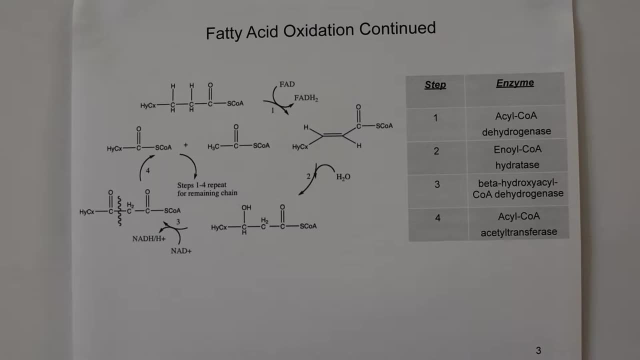 Is oxidized. Here You'll hear This spiral, Also referred To as The beta Oxidation Pathway, So don't Let that throw You off. In step three. In step four, The beta. 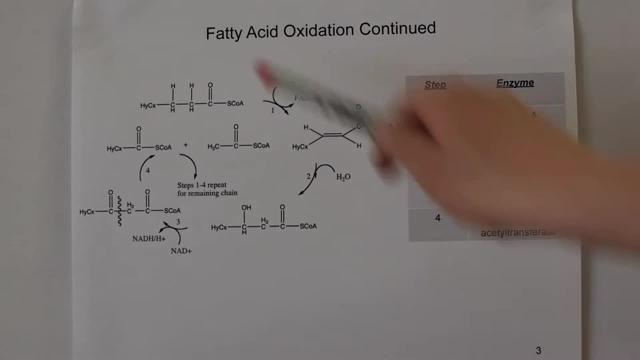 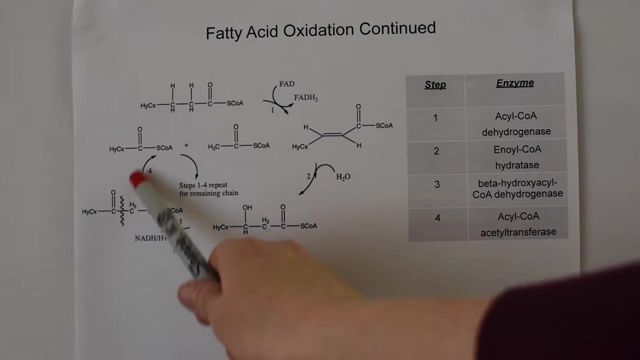 Oxidation, Fatty Acid, Spiral, Those are all Just different Ways Of referring To the same Thing, And that is These four Step, This four Step Catabolic Process That breaks. 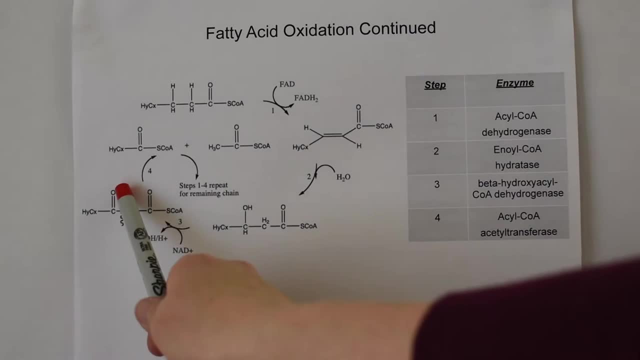 Down Your fatty Acids Into acetyl Coenzyme A. Okay, So that's A Acetyl Coenzyme A. That leaves Us With An activated Fatty Acid. That is now. 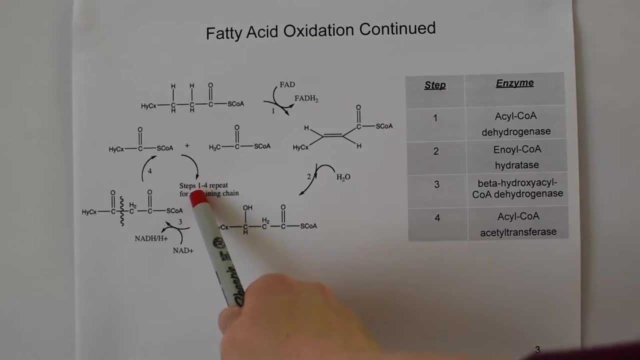 Two Carbons Shorter And it's Going To Go Back Into Step One. Re-enter The fatty Acid Spiral On Step One Now. Notice That In The last 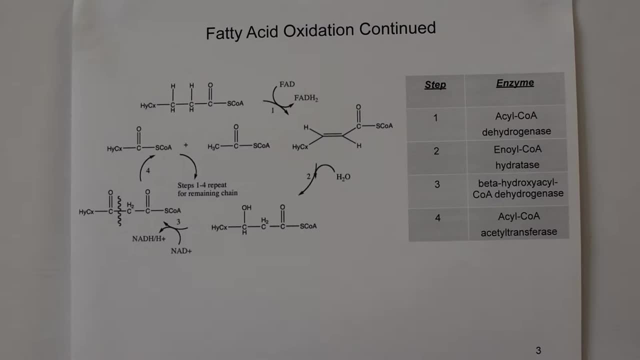 Spiral, The last Turn Of The Spiral, When You Only Have Four Carbons Left On Step Three. This Cleavage That Occurs On Step Four Is: 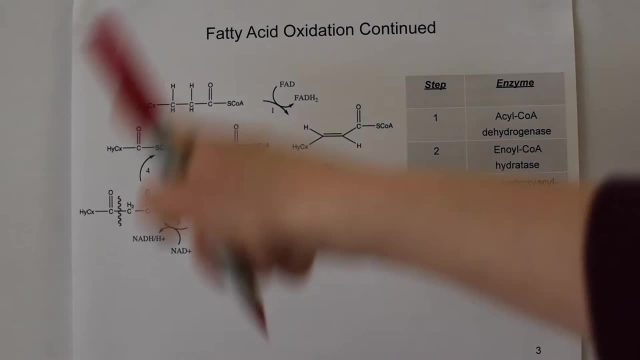 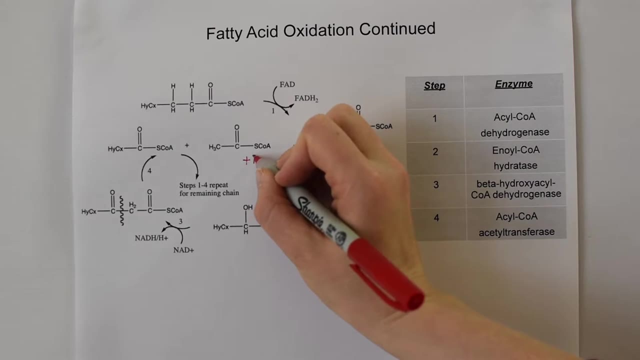 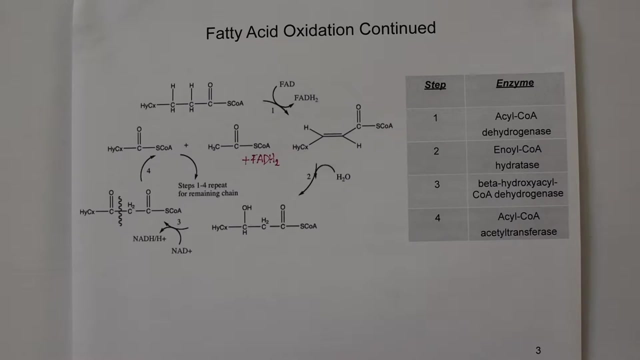 Okay, So Let's See What Do We Get From One Turn Through The Fatty Acid Spiral. Well, On Step One We Get A Reduced Coenzyme. 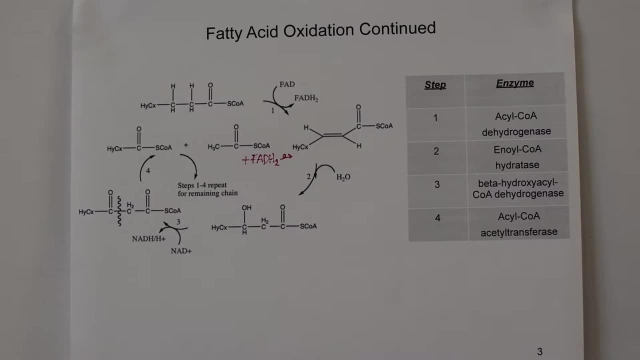 Of FADH2.. And We Get Reoxidized. They're Going To Pass Their Electrons And Hydrogen Ions Ultimately To Oxygen From The Air. 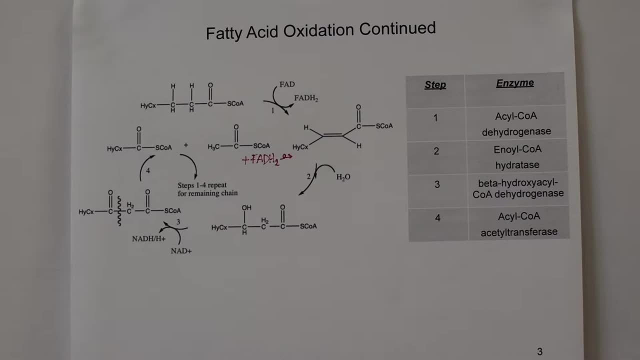 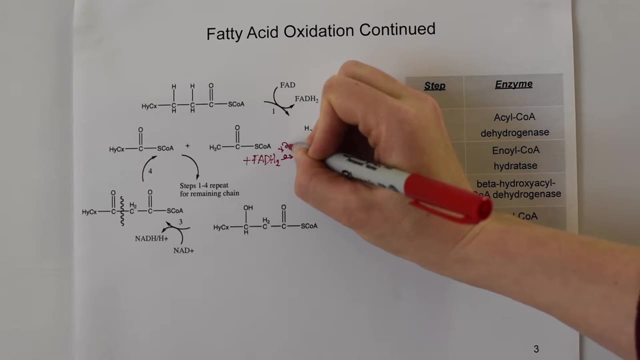 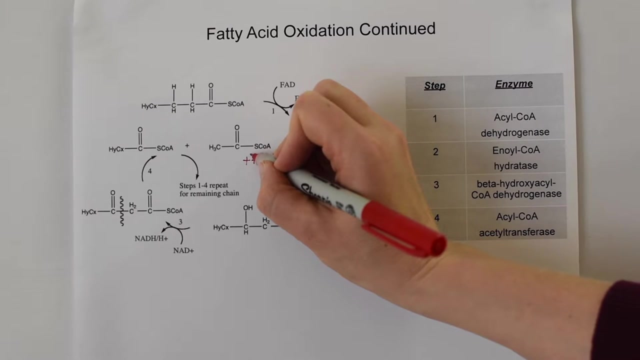 That We Breathe To Make Water And That Exergonic Process Is Going To Power The Synthesis Of Two ATPs. So, From This Process, 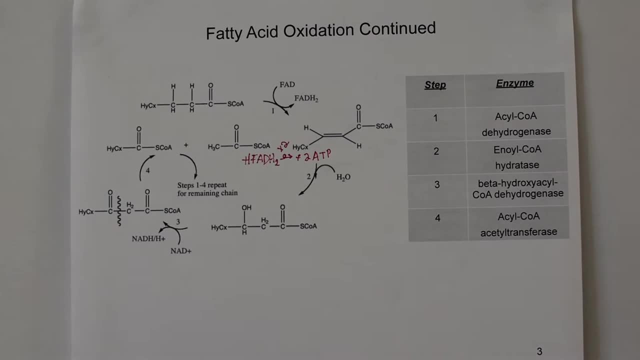 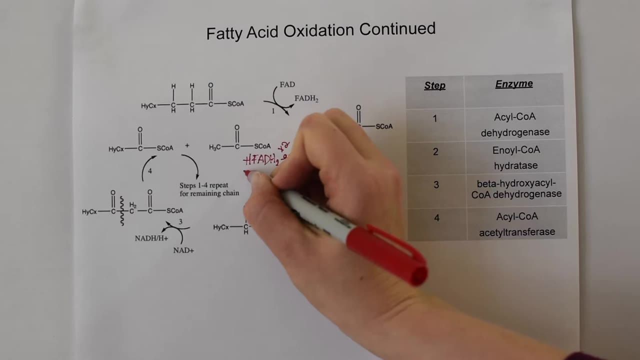 So I Should Write Plus One FADH2.. We Get Plus Two ATP Later On In The Electron Transfer Chain NADH. And Remember When. 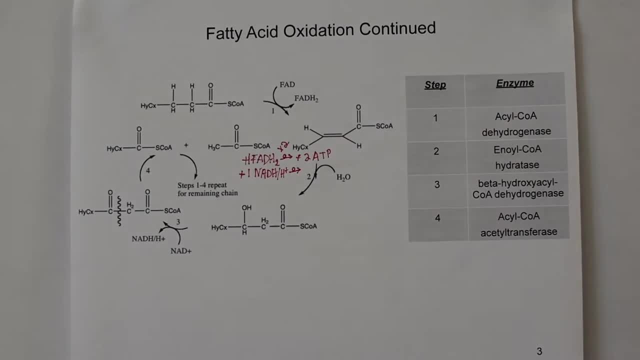 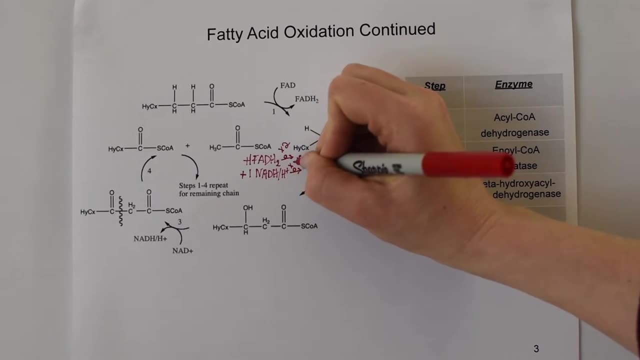 That Is Reoxidized In The Electron Transfer Chain, And Oxidated Phosphorylation For Every One NADH, We Get Three, So Times Three. 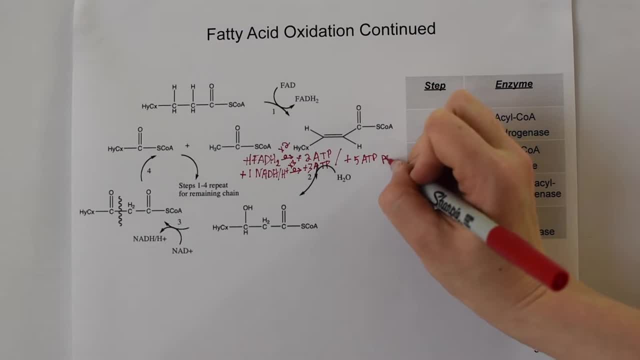 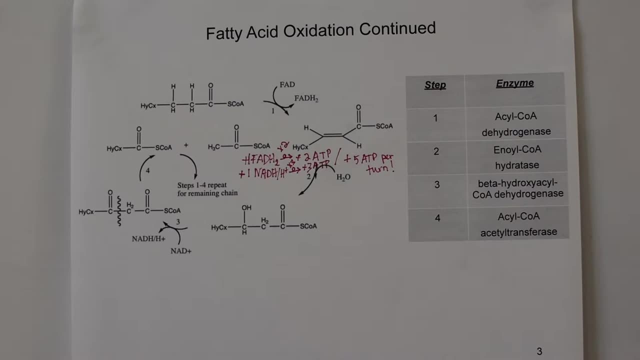 ATP. So We're Going To In The Spiral. Well, How Many Turns Do We Get In The Spiral? Think About What Your Fatty Acids. 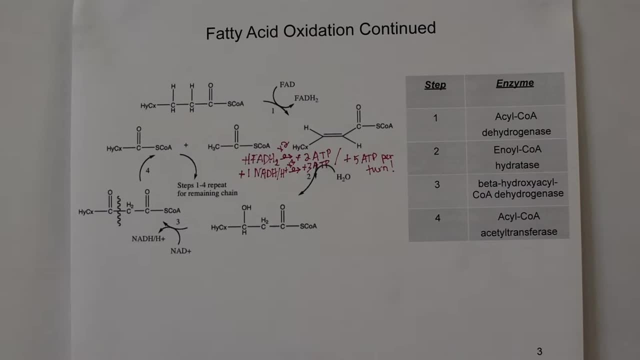 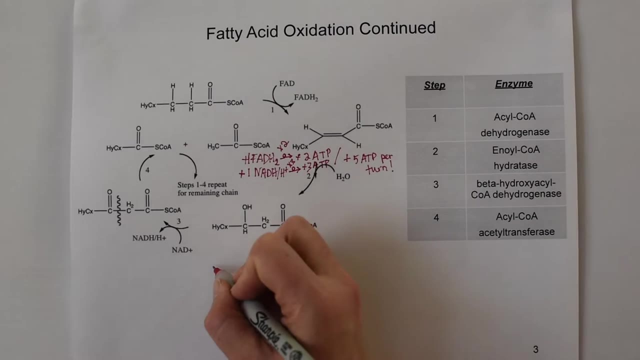 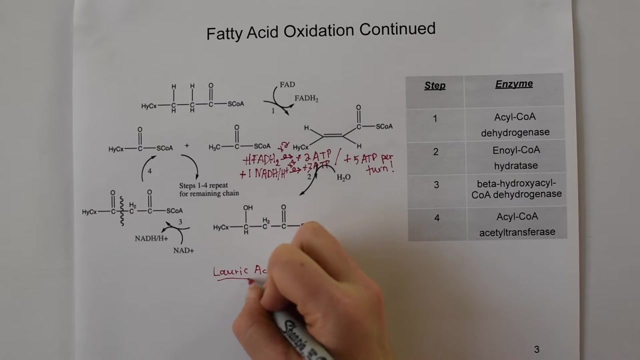 Look Like There's A Bunch Of Different Ones, Right, Some. I'll Write This Down Here, Which Is A Twelve Carbon Saturated Fatty Acid. 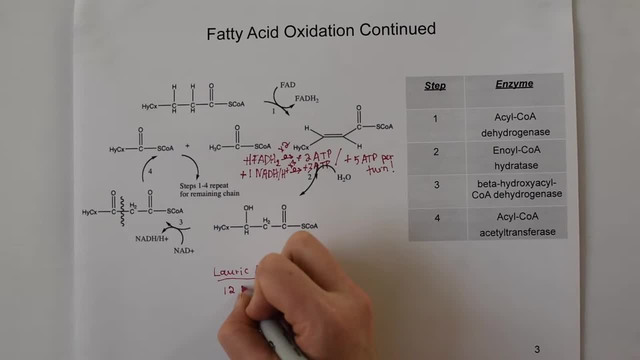 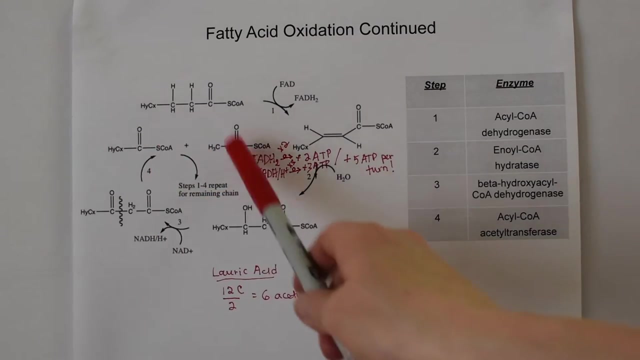 Well Then, We're Going To Get Twelve Divided By Two. We're Going To Get Six Acetyl Coenzyme A's, So You're Actually Going. 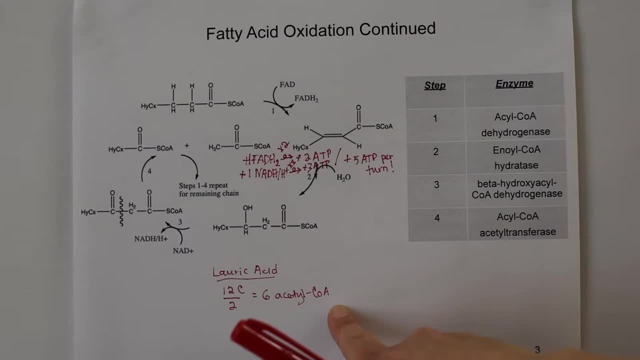 To Always Get One Fewer Turn Than The Number Of Acetyl Coenzyme A's You Make. I Hope That Makes Sense. So This Means 18.. 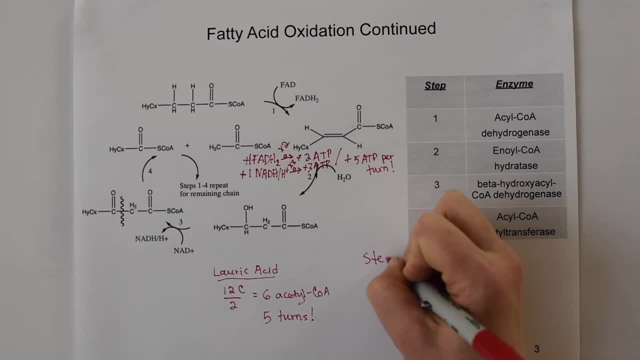 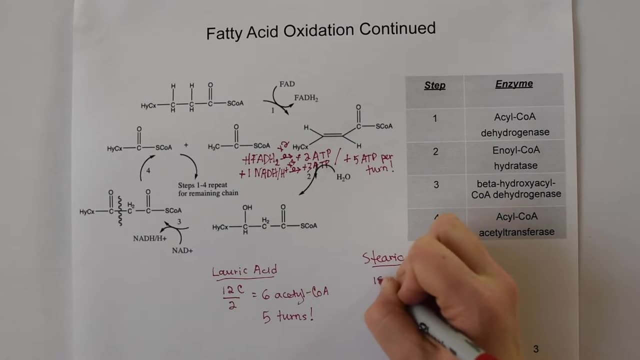 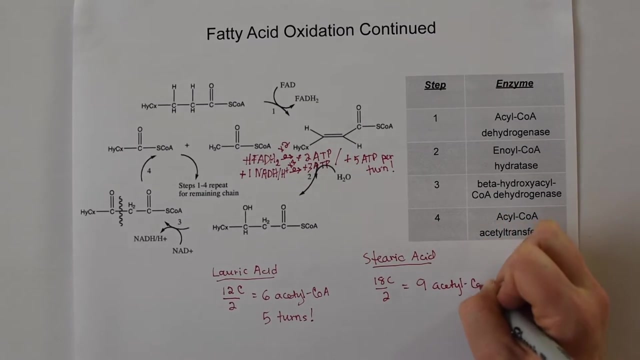 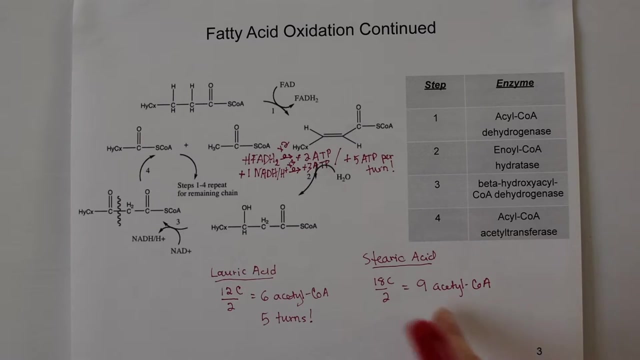 Carbon Saturated Fatty Acid, Then We'd Get 18.. Divided By Two, We Would Get Nine: Acetyl Coenzyme, A Molecules, And Since The 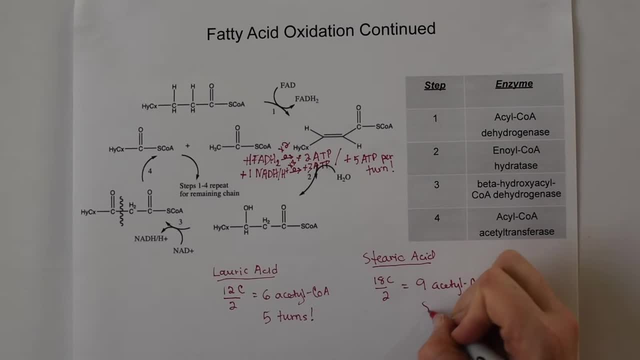 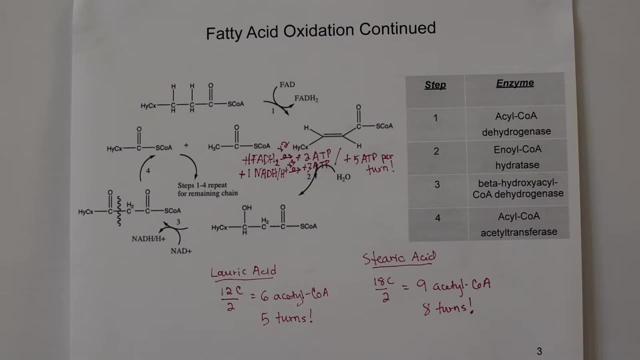 Last Turn Makes So We Would End Up Getting Eight Turns In The Spiral From Steric Acid Because It Is A Longer Fatty Acid. Okay. 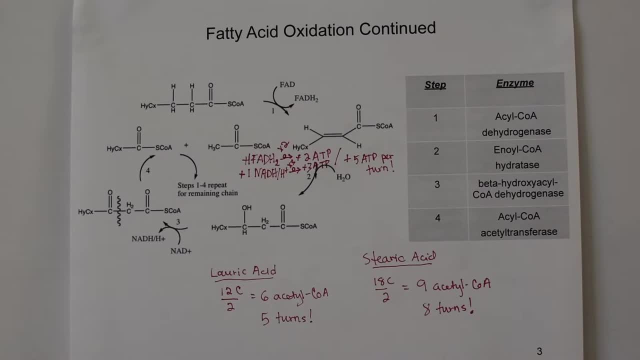 So That's What I Mean When You Get In The Spiral, But You Need To Times That By The Number Of Turns That You're Going. 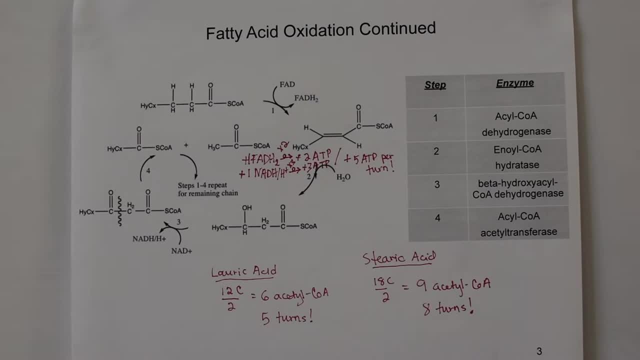 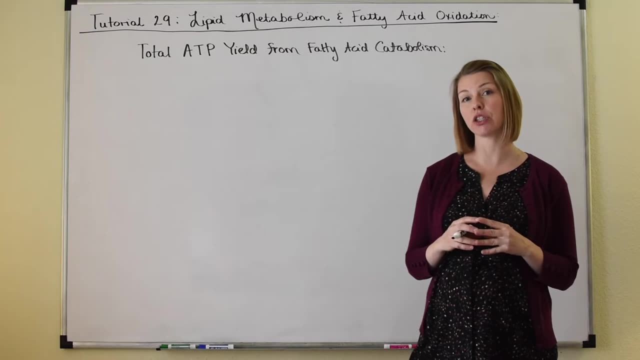 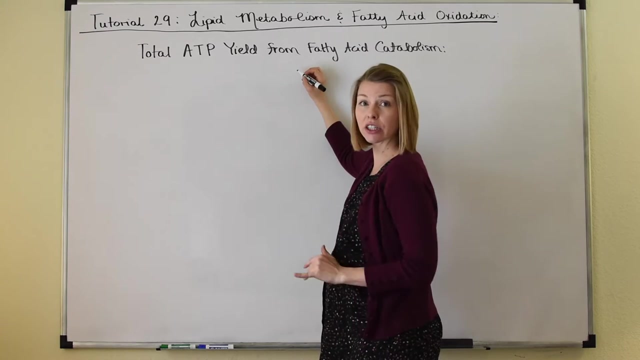 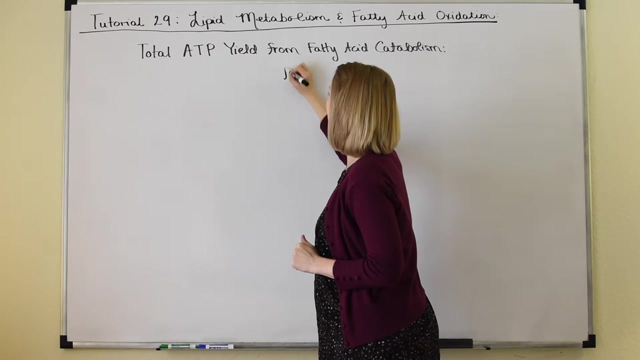 To Get In The Spiral. All Right, So Let's Go To The End Of Our Fatty Acid. Well, We Have To Count For The Entire. 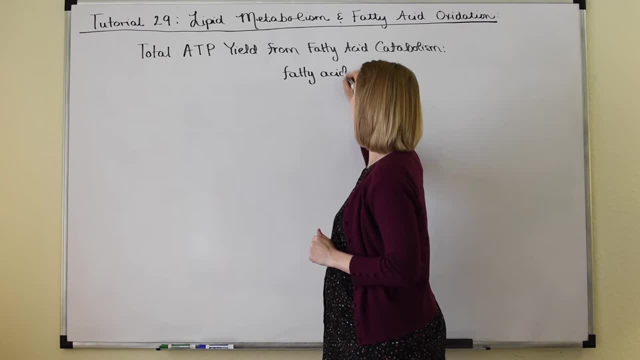 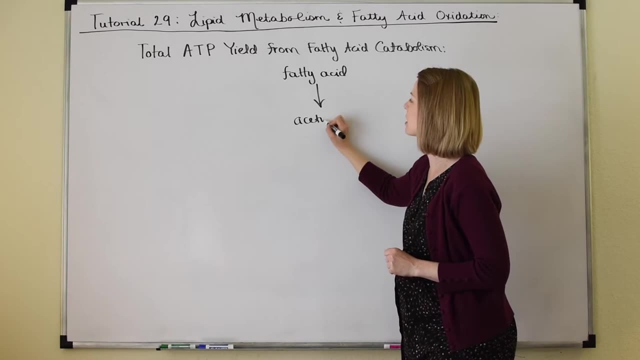 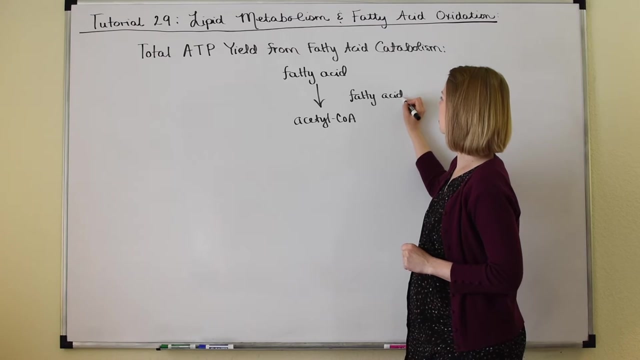 Catabolic Process Converting All The Carbon Hydrogen And Oxygen Into Carbon Oxide And Water. All Right, Fatty Acid Oxidation To Keep It. 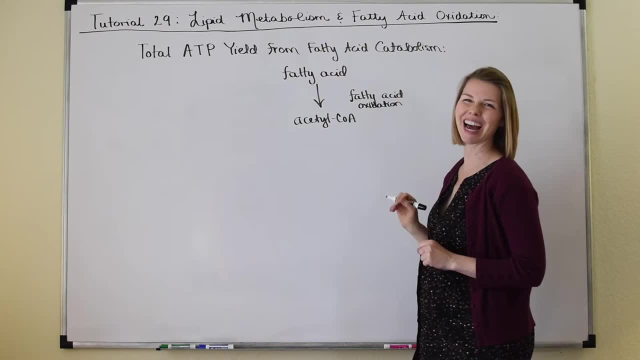 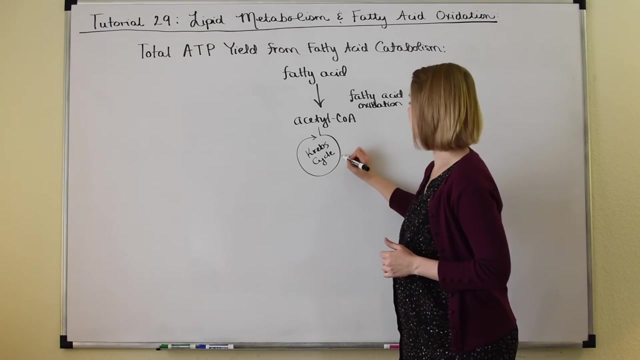 Consistent With My Title Here. And Then We Have To Count For That Acetyl Co Enzyme A Entering Into The Krebs Cycle One. 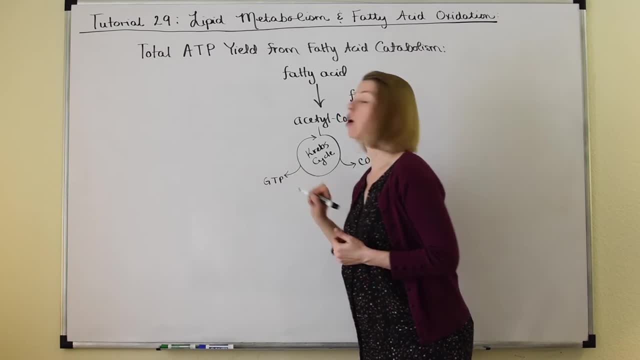 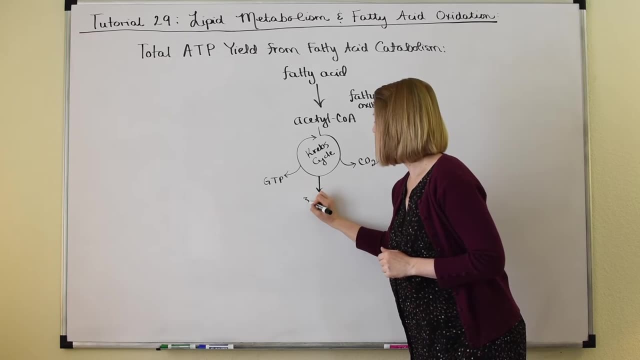 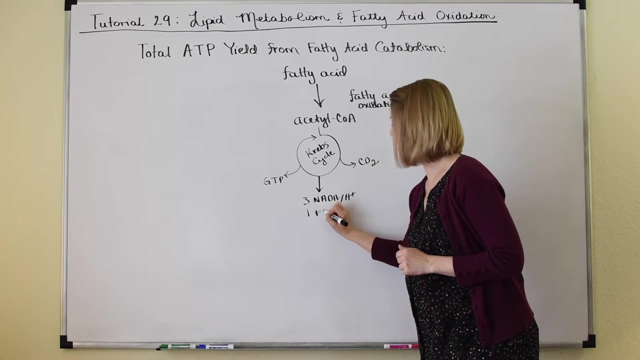 Turn In The Krebs Cycle Also Gives Us A High Energy Molecule. You Want To See Tri Phosphate And Because Overall It's Oxidation. 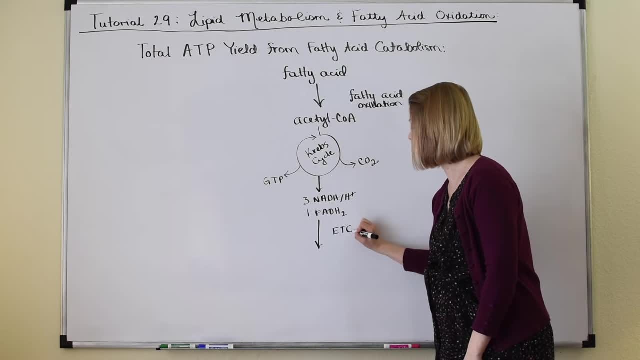 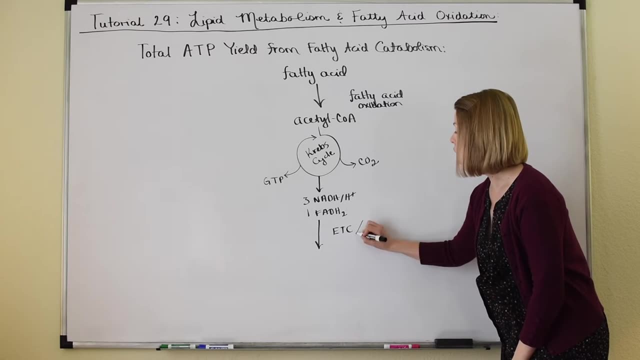 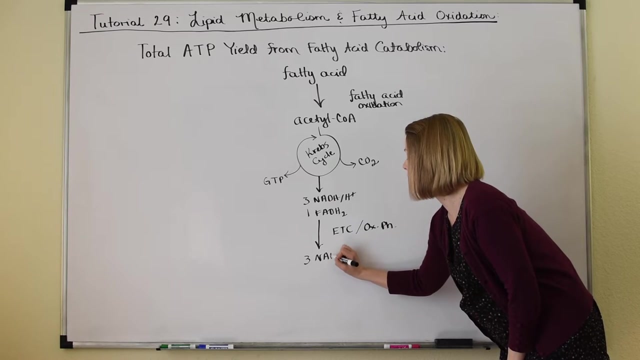 We Know Co Enzymes Get And It's The Energy Released From The Electron Transport Chain That Will Be Harnessed To Power Oxidative. 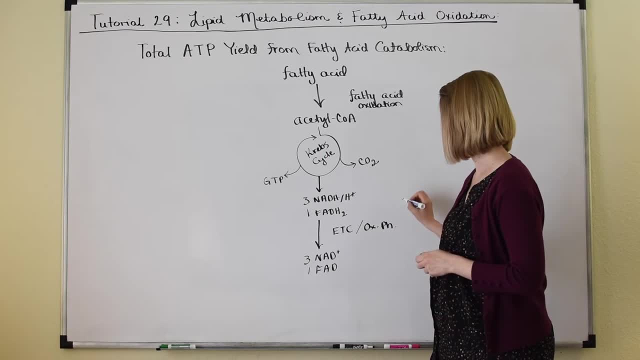 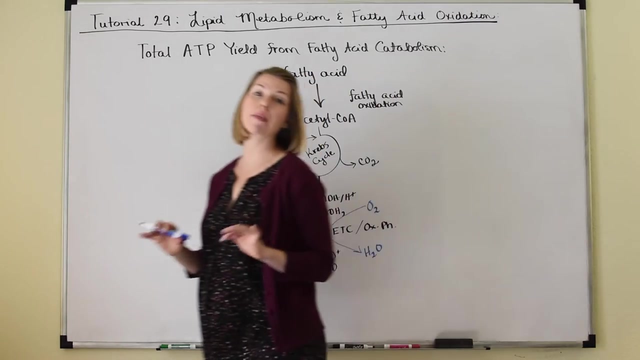 Phosphorylation. Okay, So We Get Three Reoxidized Co Enzymes Of NAD+, One From The Air That We Breathe, Creating H2O. 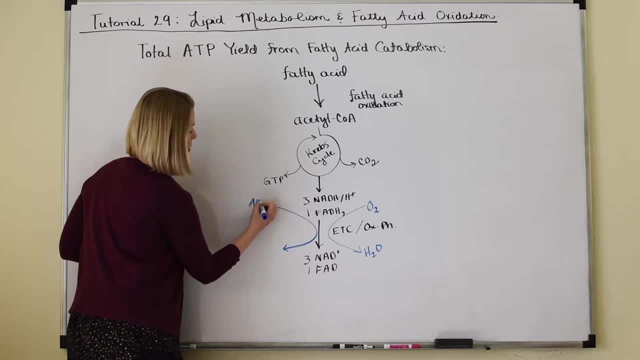 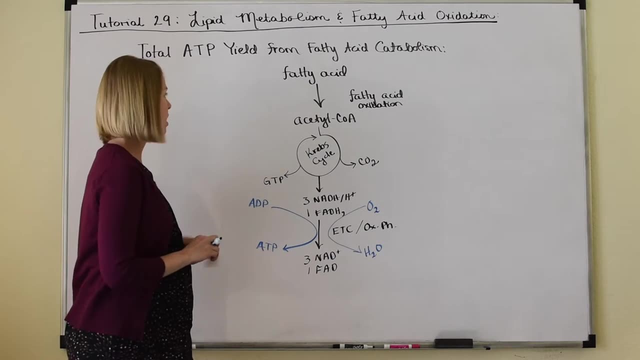 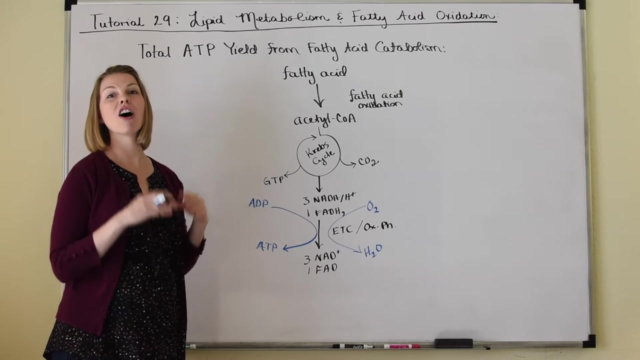 The Energy From That Extraconic Process Is Harnessed To Phosphorylate, ADP, Making ATP In The Process Known As Oxidative Phosphorylation. 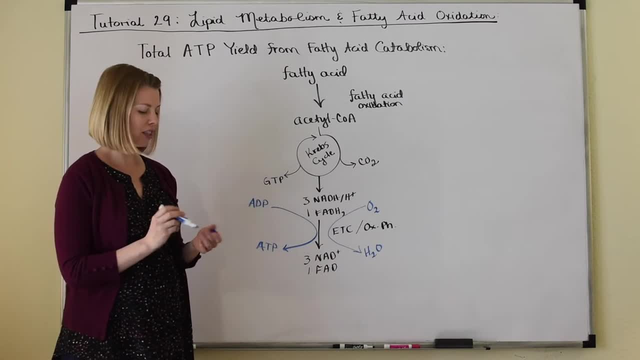 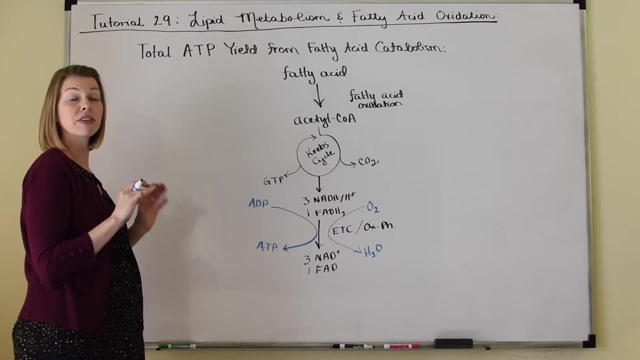 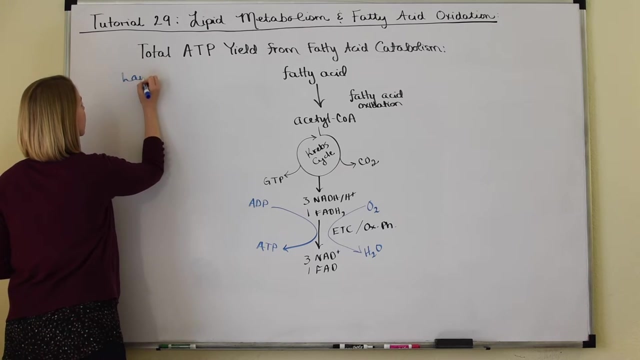 All Right, So Let's Go Ahead And Do That. We'll Stick With The Blue Pin Here And We're Going To Do It For The. 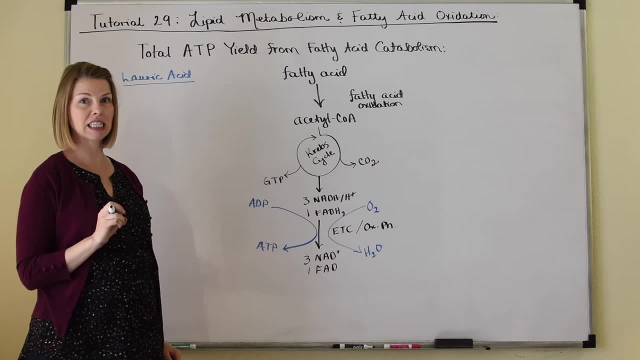 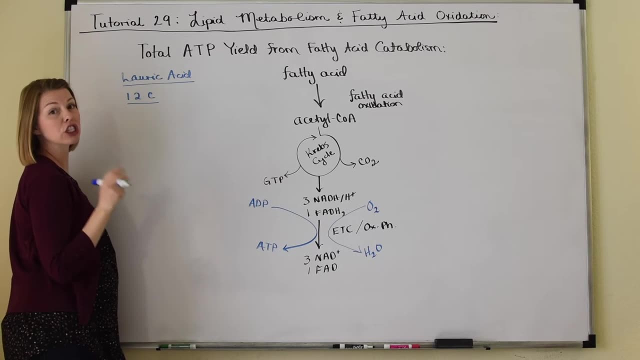 Two Fatty Acids That We Mentioned. That Is Going To Be Broken Down Into The Two Carbon Acetyl- Portion Of Acetyl Coenzyme. 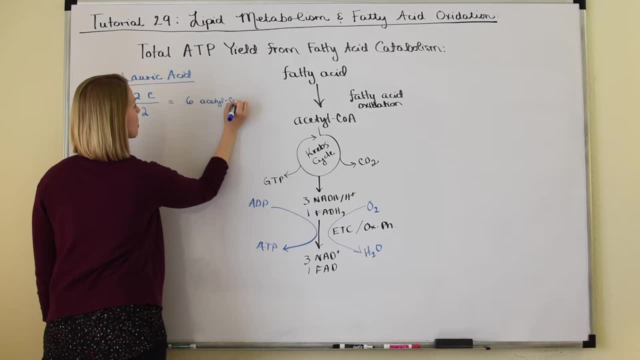 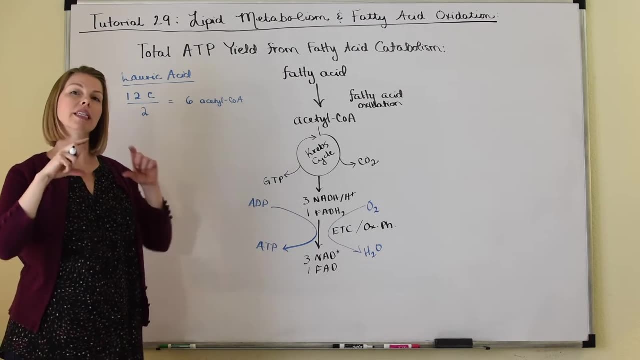 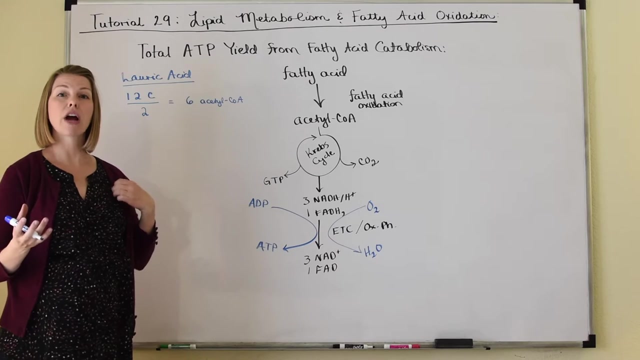 A, So Divide By Two And Figure Out How Many Acetyl Coenzyme A's And Cleave Them Into Two Acetyl Coenzyme A's All. 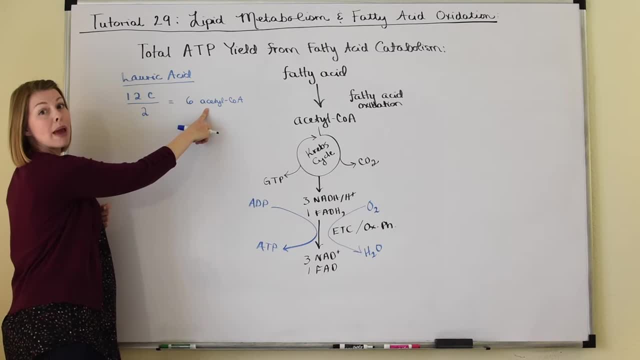 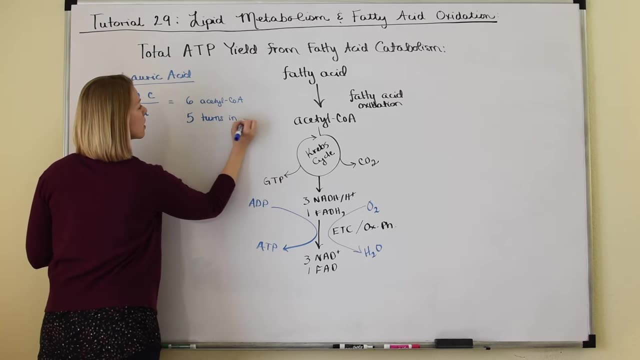 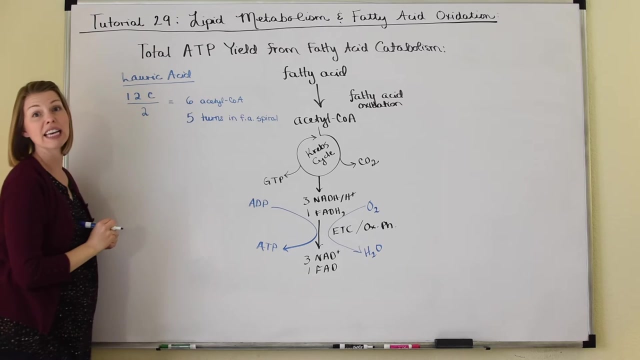 At Once. So You're Actually Going To Get One Fewer Turn In The Spiral Than The Number Of Acetyl Coenzyme. All Right, So You. 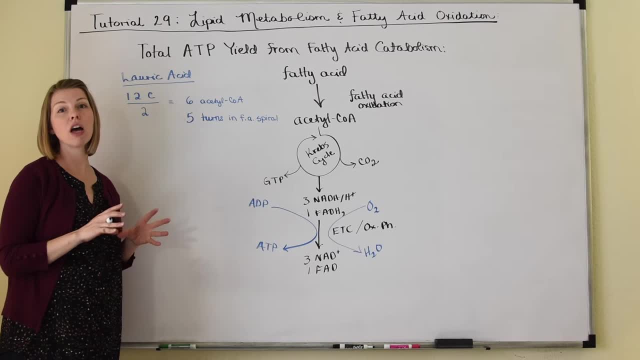 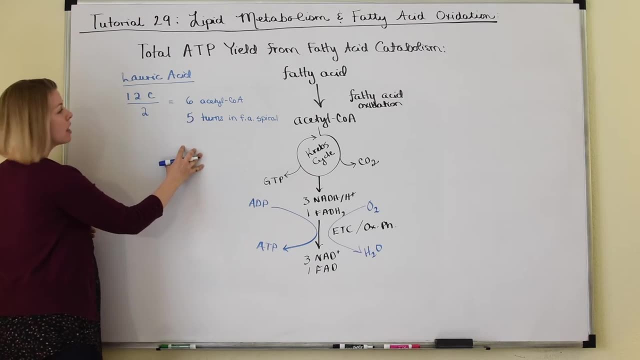 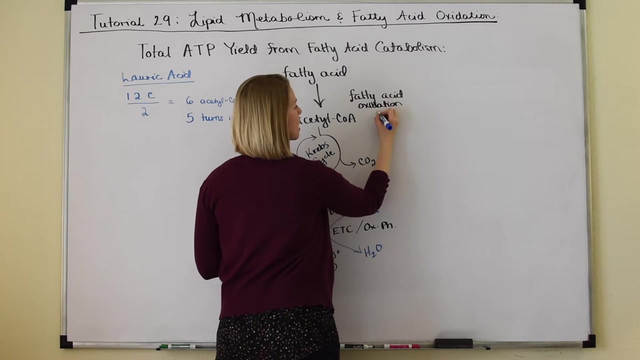 Can Look At The Fatty Acid Spiral On Slide Three If You Need To Remind Yourself Of The Steps That Are Happening There And 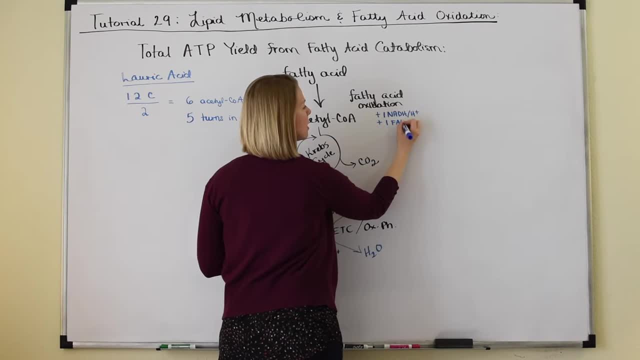 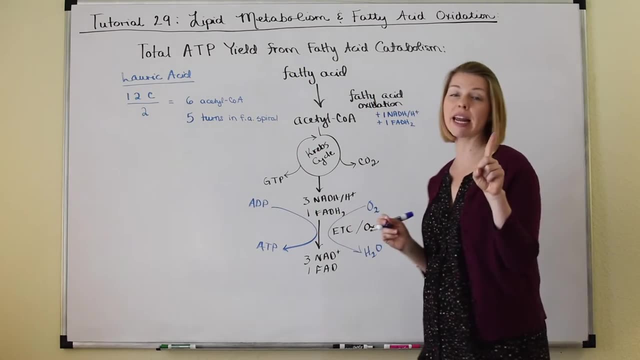 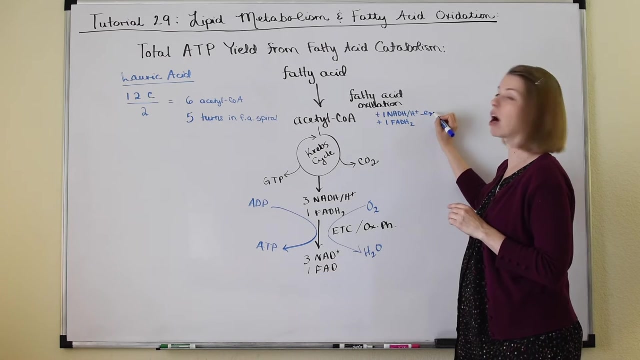 Where We Are Going To Get One F, A, D, H, Two, Okay. So When NADH Gets Reoxidized, Remember That For Every One NADH. 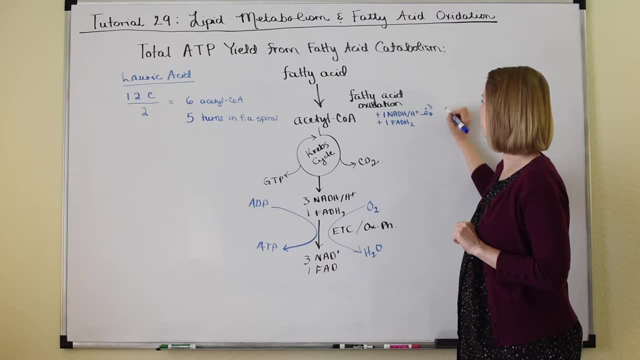 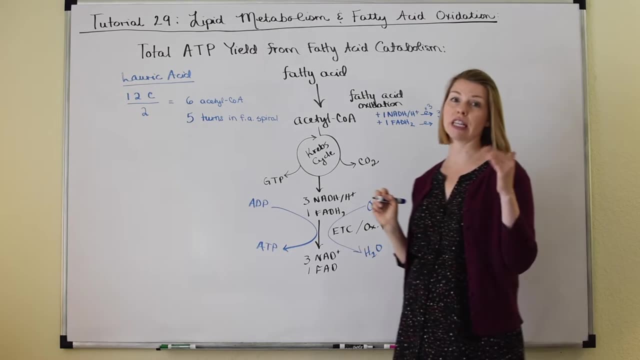 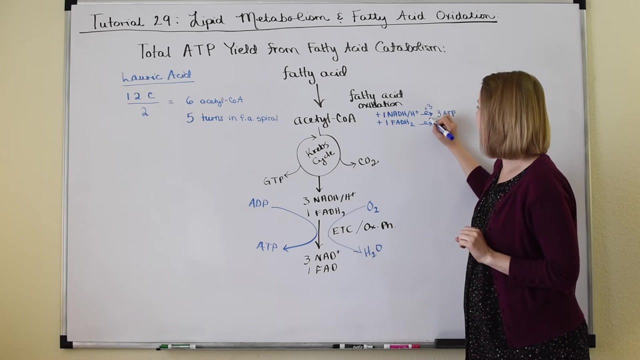 You're Going To Get Three ATP. Remember That F, A, D, H, Two Enters The Electron Transport Chain Later, Giving Us Less Energy And Therefore, 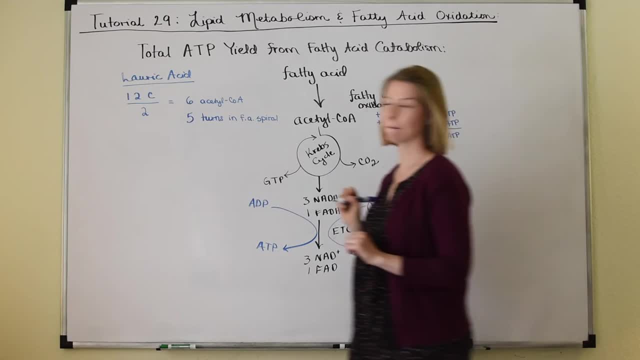 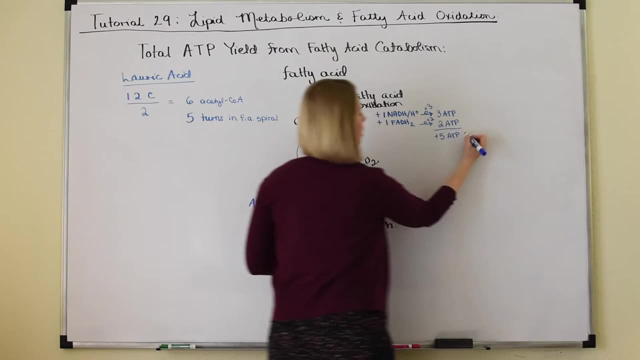 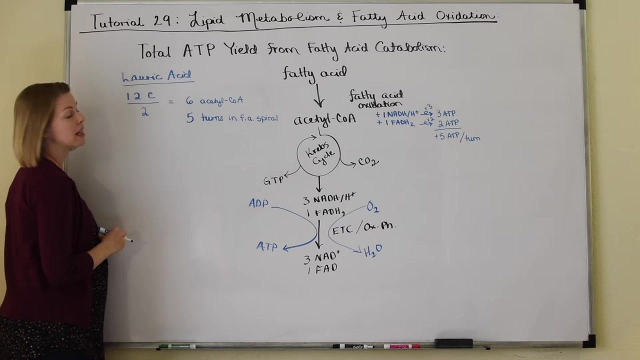 Creating Less ATP. So We're Going To Times That By Two Per Turn In The Spiral And There Are Five Turns In The Spiral To 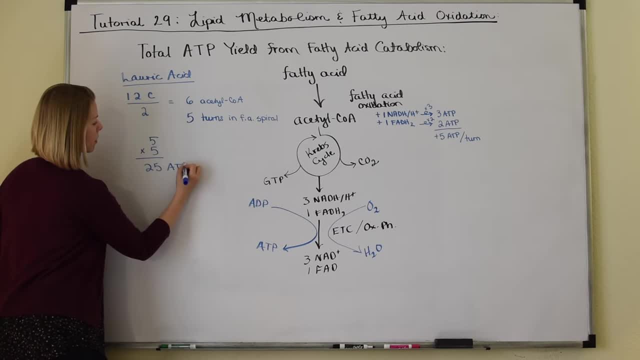 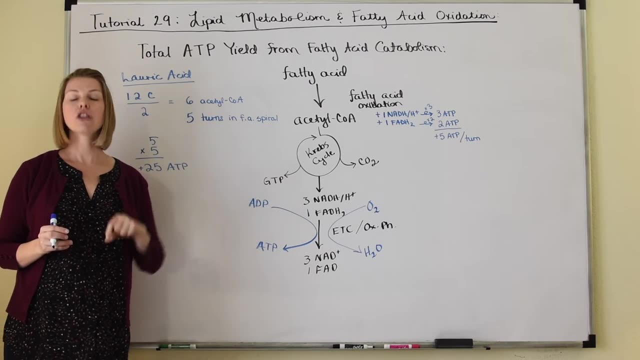 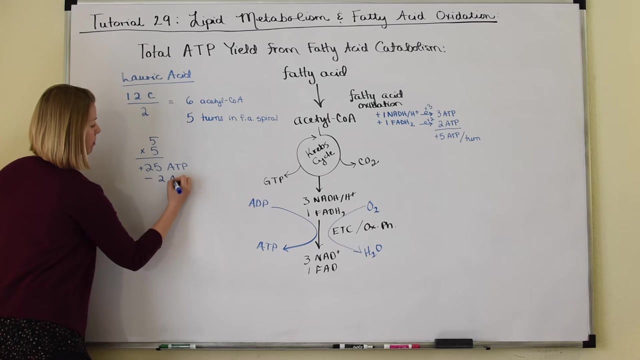 Catabolize Galoric Acid. That Gives Us Five Times Five. That Gives Us Twenty Five ATP. So We're Going To Subtract That Two Here. 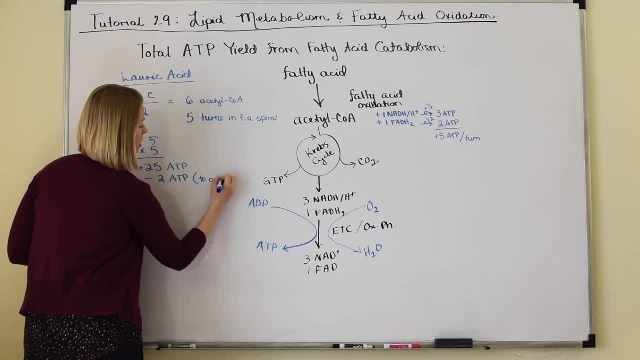 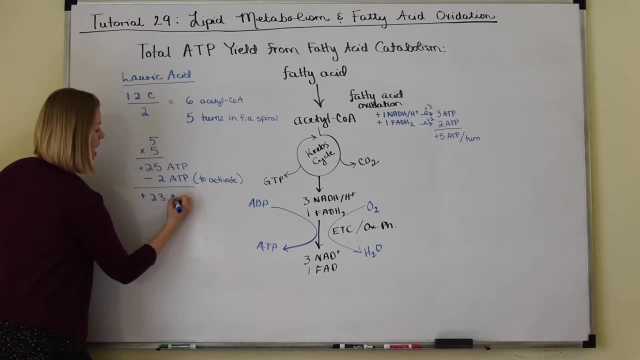 And I'm Going To Put A Little Reminder Here Of Why I'm Doing This: Minus Two ATP To Activate, That's To Turn The ATP. 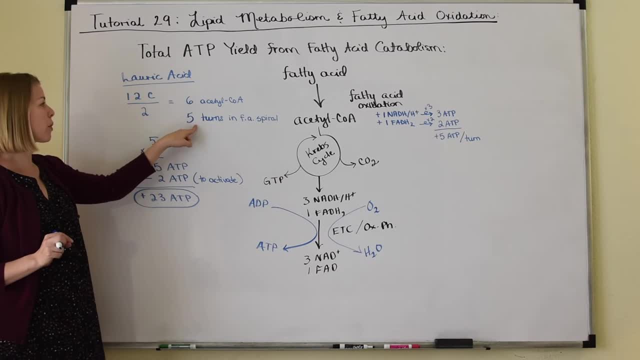 That I Get From Reoxidizing The Reduced Coenzymes That Were Created In The Five Turns Of The Fatty Acid Spiral. Notice We Also 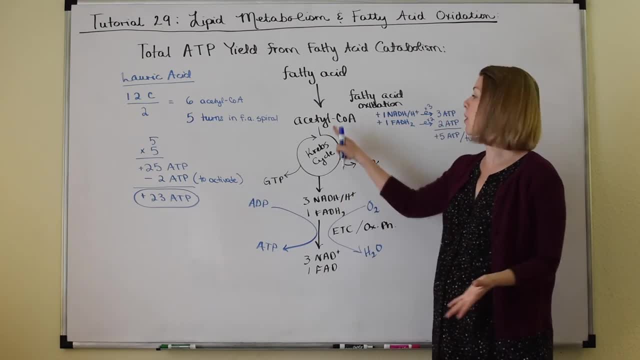 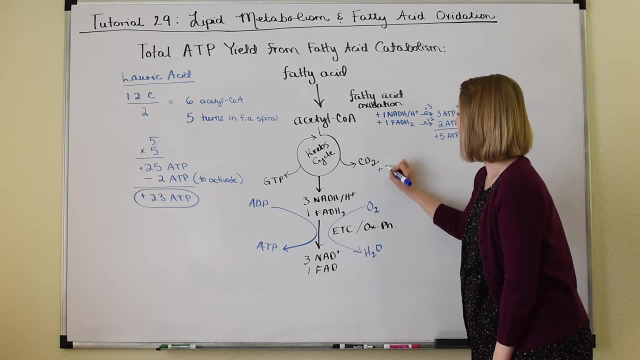 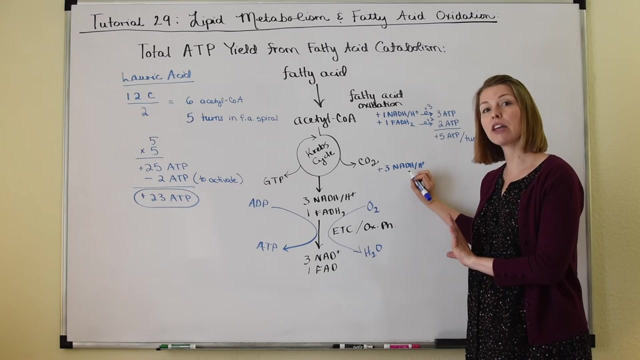 Have Six Acetyl And We Get Per Turn In The Krebs Cycle. We Know That We Get And It's Really All Summarized Here. 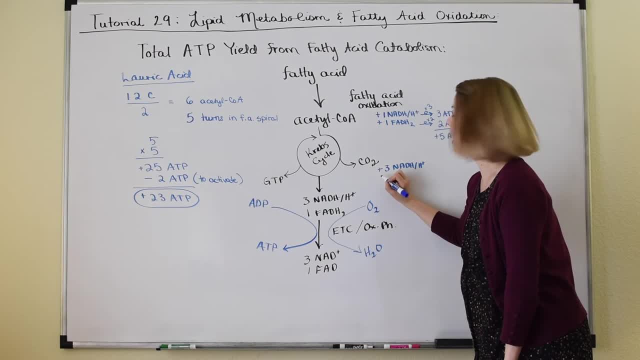 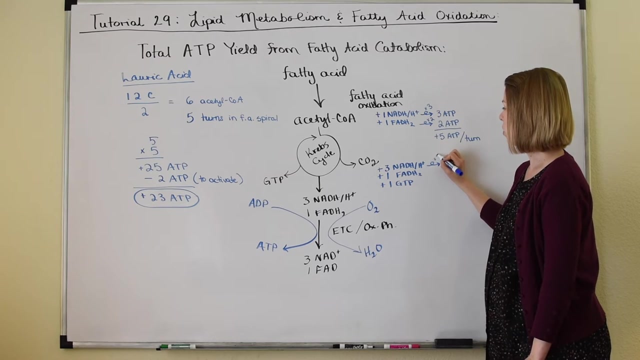 Already For Us. We Get Three Reduced Coenzymes Of The One High Energy GTP Molecule. Okay, So That Means That Later On, When These 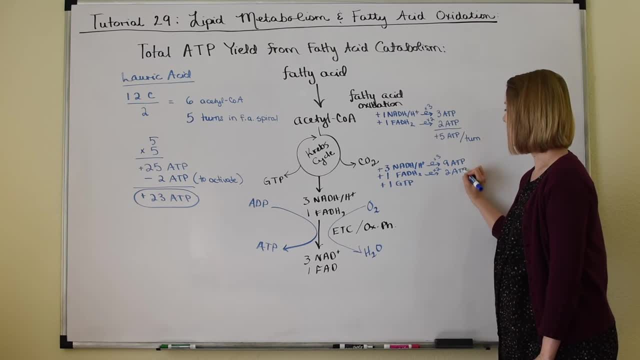 Are Reoxidized In The Electron Transport Chain, We're Going To Get Three Times Three, So Plus Twelve ATP Per Turn In The Krebs Cycle. 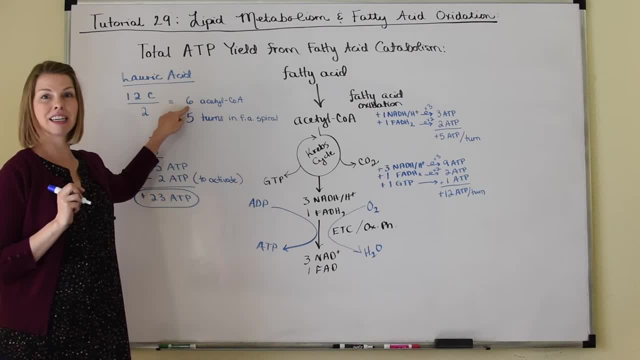 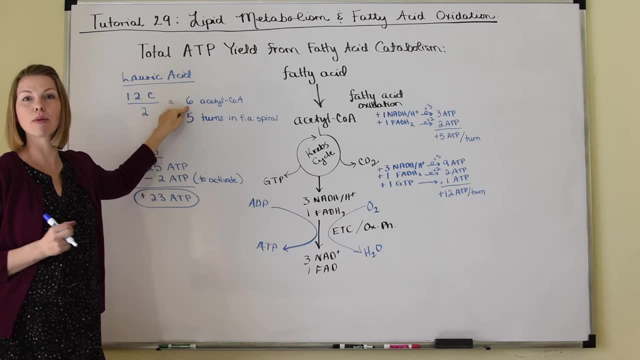 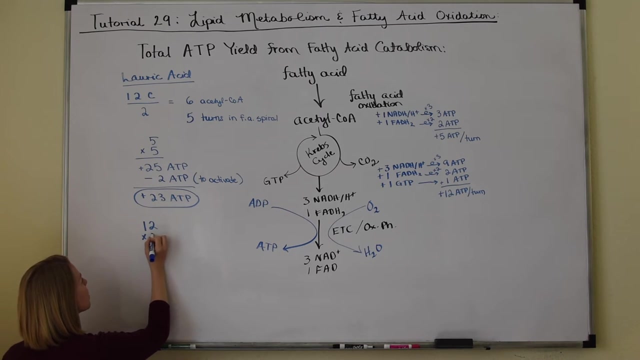 Okay, Well, How Many Turns Do We Get In The Krebs Cycle? We're Going To Get Six, Because All We Have Seventy Two Plus. 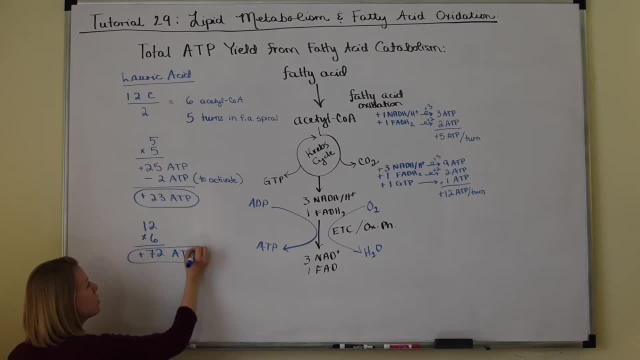 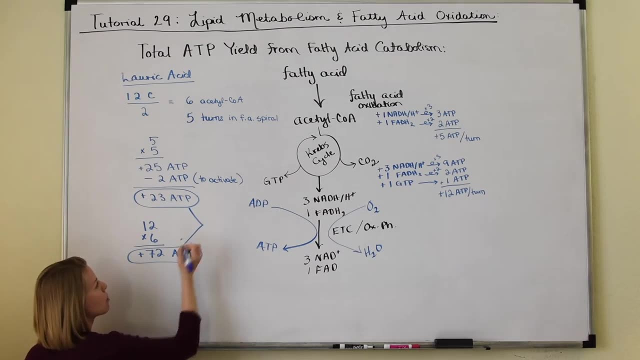 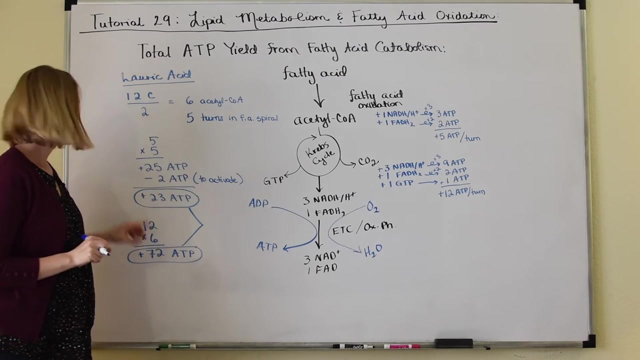 Seventy Two ATP. I'm Going To Circle That Two, Okay, And Then If We Want To Find Out Our Total ATP Yield, We Need From: 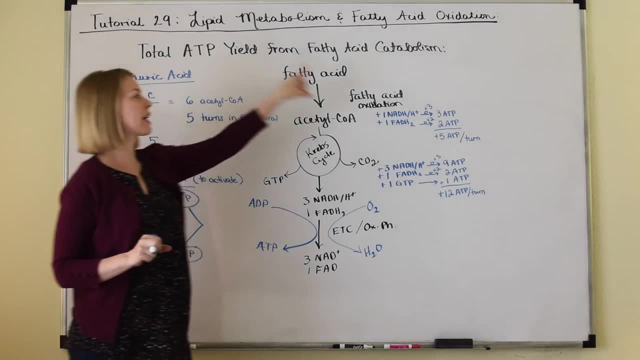 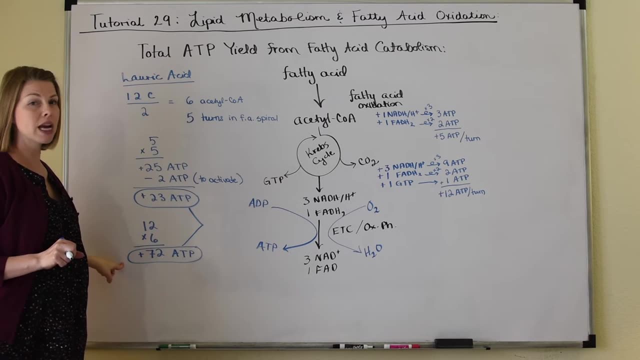 The Reoxidation Of The Reduced Coenzymes That Came From The Fatty Acid Oxidation. Remember That The Plus Seventy Two Came From Complete 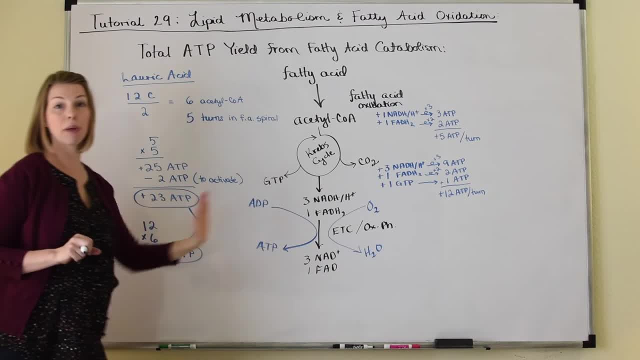 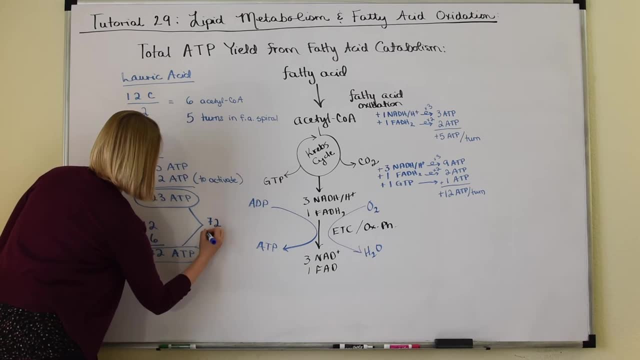 Catabolism Of The Six Acetyl Coenzyme A's Together Gives Us Seventy Two Plus Twenty Three, Ninety Five ATP. That's Your Final. 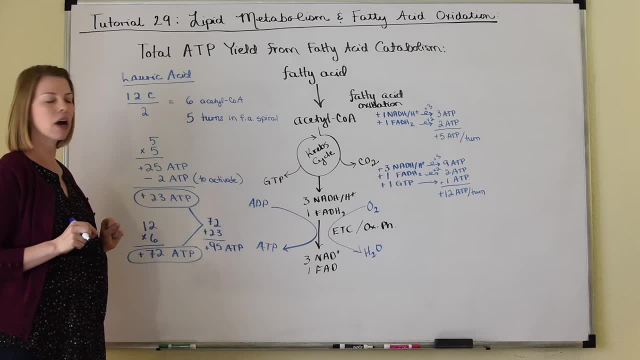 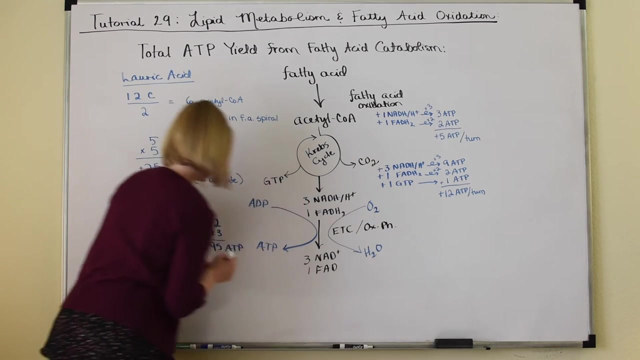 Answer: So For One Little Molecule Of Lauric Acid Being Completely Catabolized, We Can Get Ninety. So Let's Circle That In The 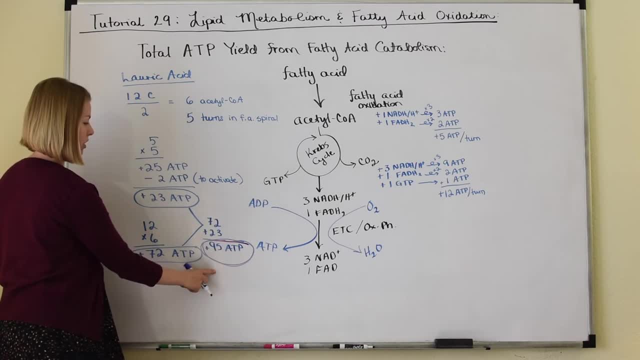 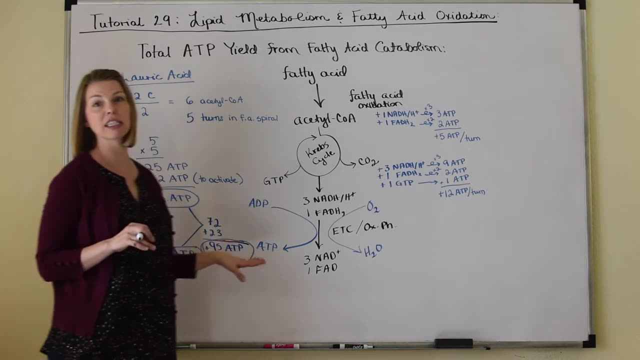 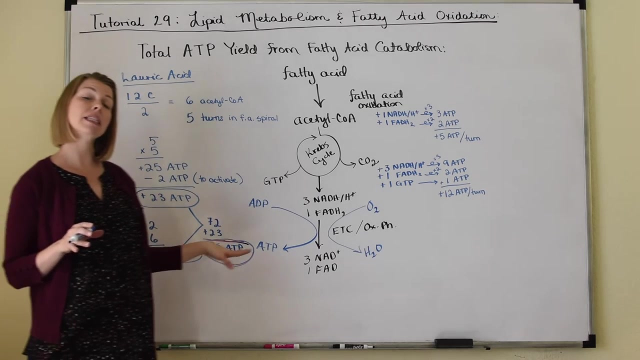 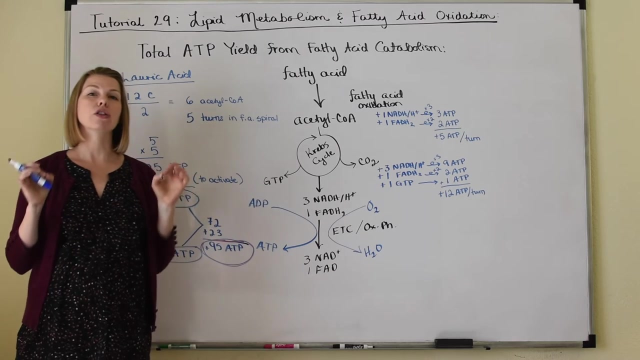 Pink And The Blue. I Really Want That Final Answer To Stand Out There. Okay, So That's Our Final Answer. So Real Quick, So We. 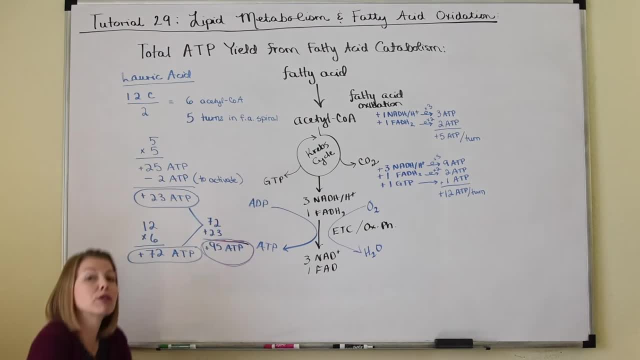 Did A Total ATP Yield For Complete Catabolism Of Glucose. For Every One Molecule Of Glucose That's Completely Catabolized, We Said 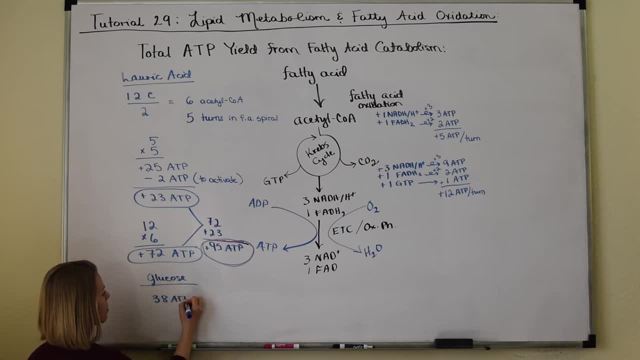 Glucose. Here We Get 38. ATP. Okay, Actually, Let's Write It Like This: 38. ATP Per Every Glucose Molecule We Just Said For. 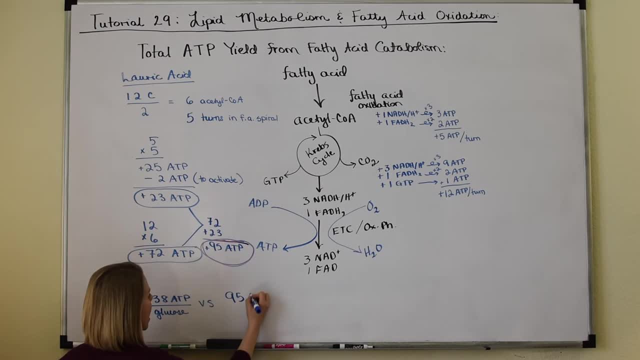 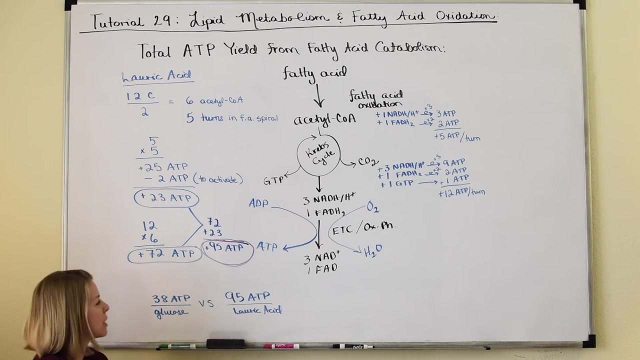 A Similarly Sized Fatty Acid- Lauric Acid- That We Get 95. ATP For Every, Two Times The Energy That We See For The Complete. 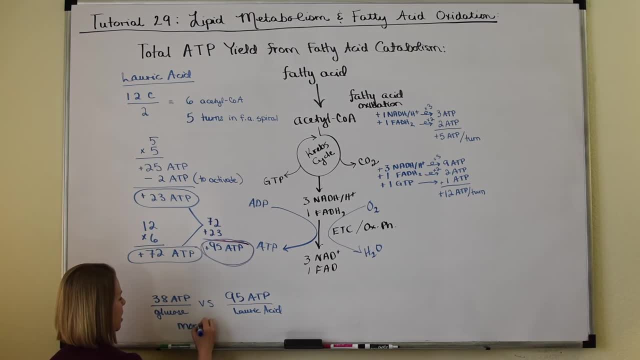 Catabolism Of The Fatty Acid Versus The Similarly Sized Glucose Molecule. So Let Me Write Here More Than Two Calories, Okay, And 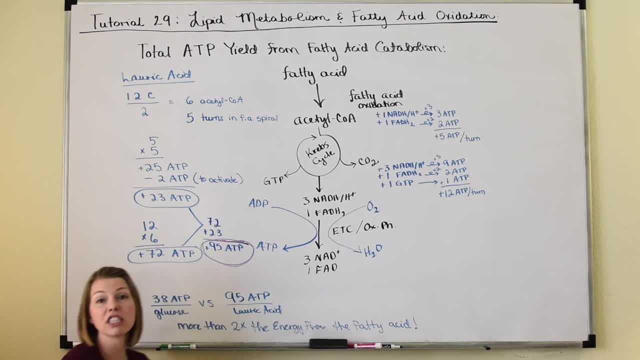 If You've Taken Nutrition, You've Probably Already Seen This Represented In Terms Of Nutritional Calories, So You Probably Already Know That You Get Four. 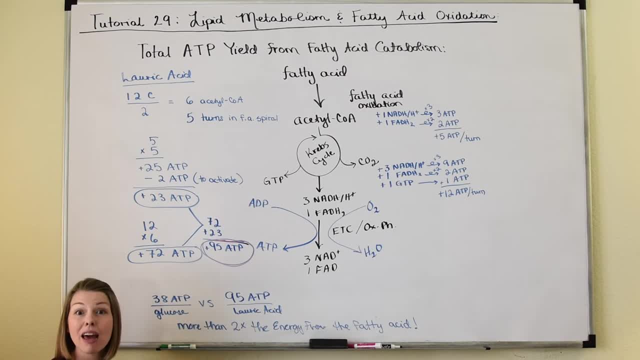 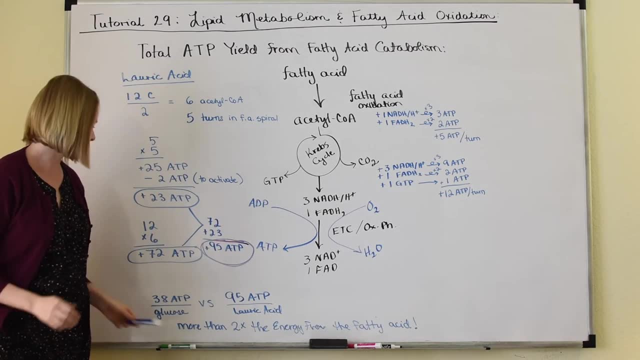 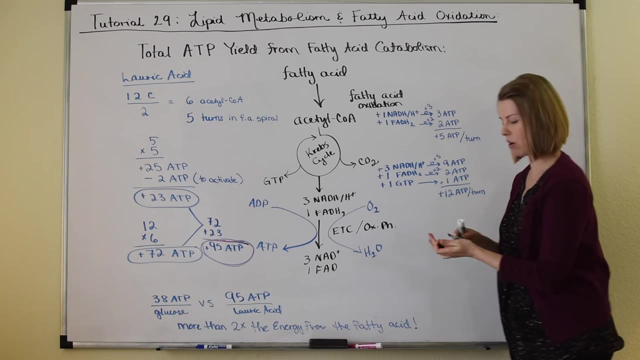 Nutritional Fats That You Eat. So Again, More Than Two Times The Energy For The Same Quantity Of Food. All Right, So Let's Go. 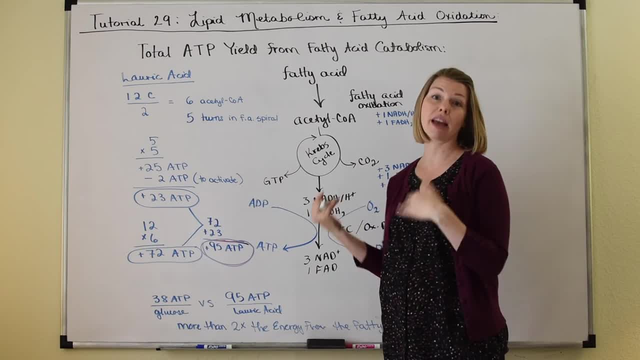 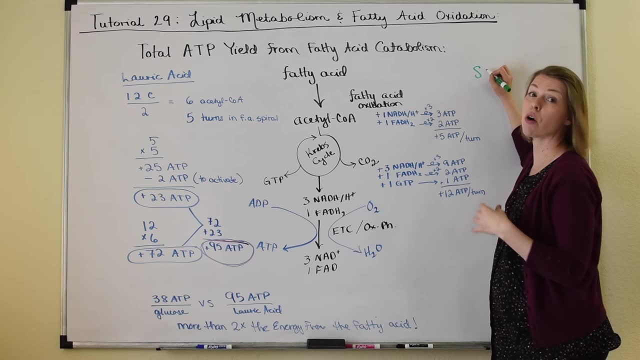 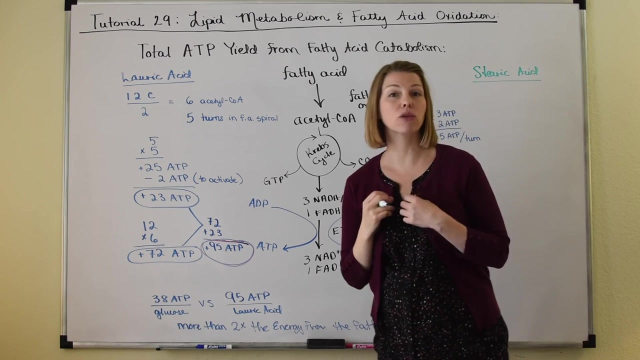 Ahead And Let's Turn To The Spiral. So It's Kind Of Nice To Do Both As Examples And See How The ATP Yield Really Is. 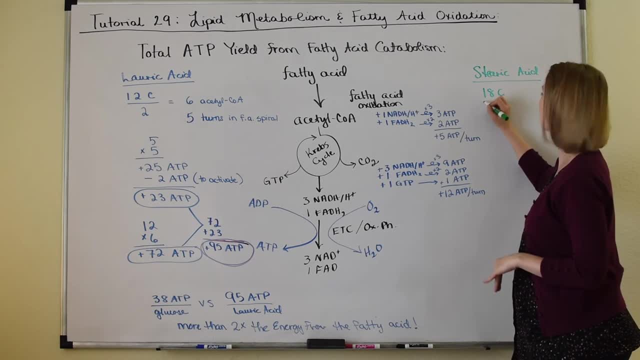 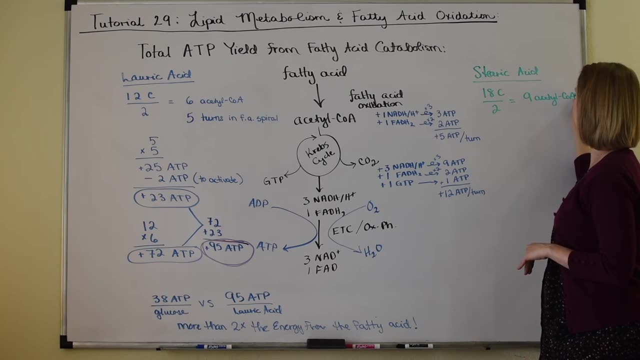 Going To Vary Because The Number Of Carbons In Your Body, Which Means We're Going To Get One Fewer, Turns In The Fatty. 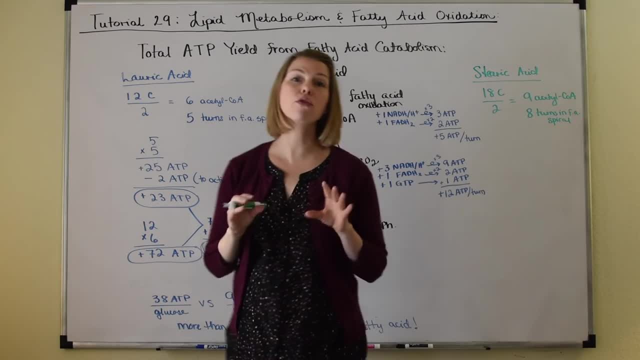 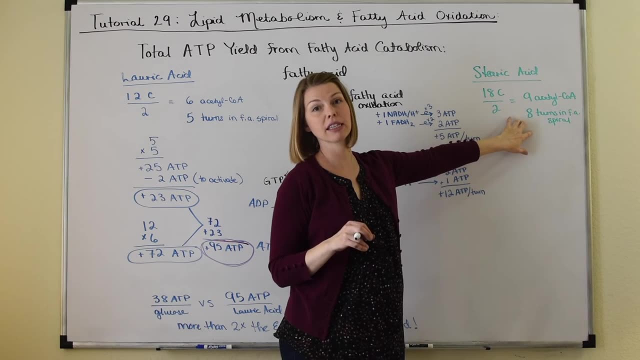 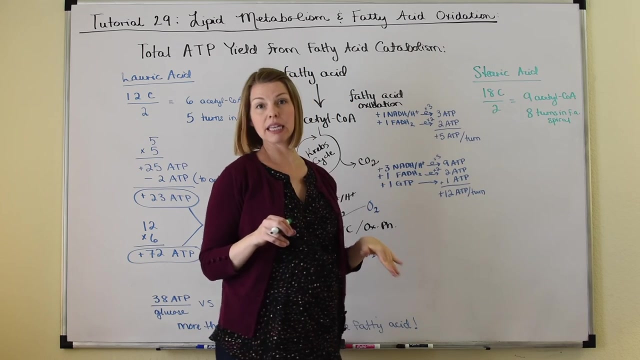 Acid Spiral, All Right. So We Need To Account For The Energy That We're Going To Get To The Carbs And Be Completely Catabolized. 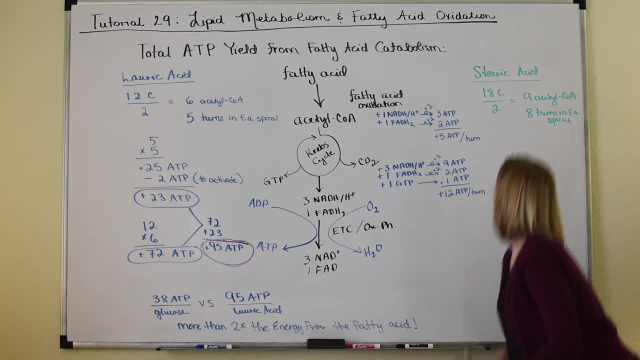 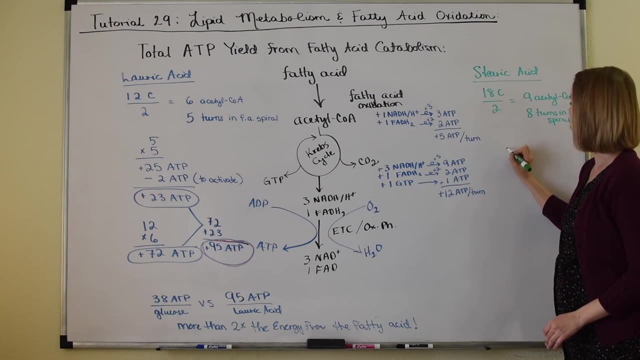 In The Krebs Cycle Electron Transport Chain Empowering Oxidative Phosphorylation, Just Like We Did Over There. So We're Going To Get Those. 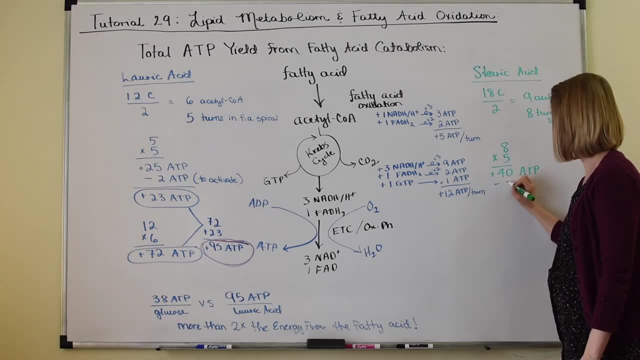 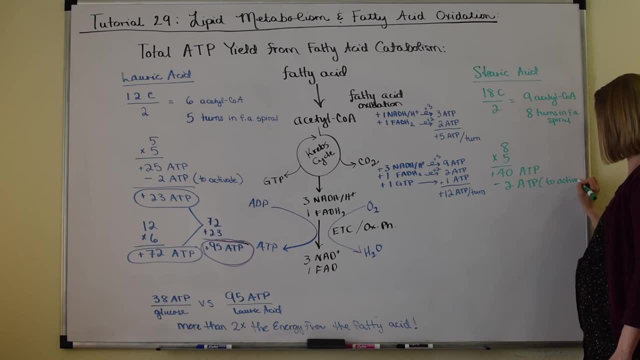 Minus Two ATP, And I'll Remind You Here. This Is To Activate, And That's Just So That The Fatty Acid Can Enter Fatty. 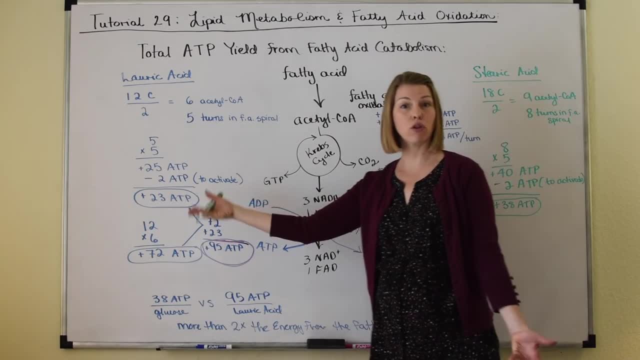 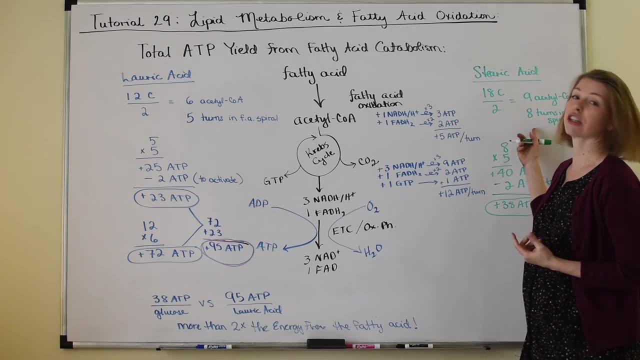 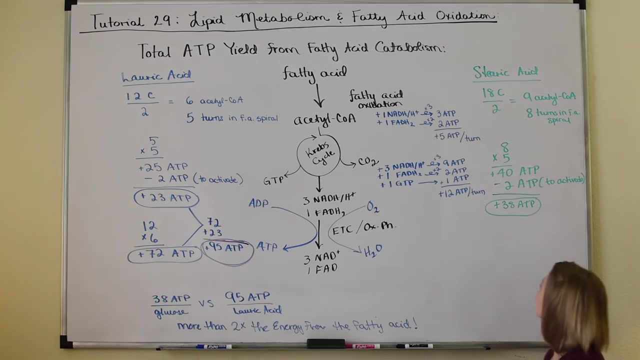 Acid Oxidation In The First Place Is A Longer Chained Fatty Acid. So We Got More Turns In The Spiral Because We Had To. 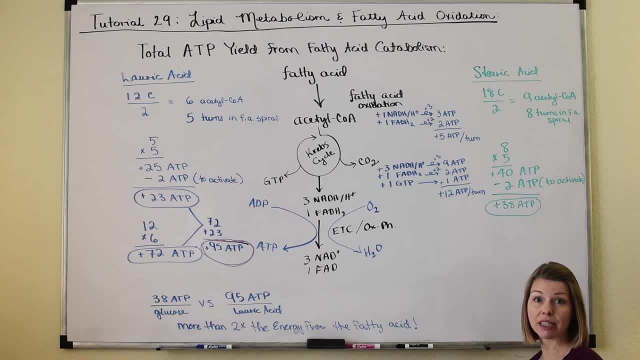 Break Down More Carbons Into More Acetyl Coenzyme A's. All Right Per Turn In The Krebs Cycle, But We Don't Just Have 12.. 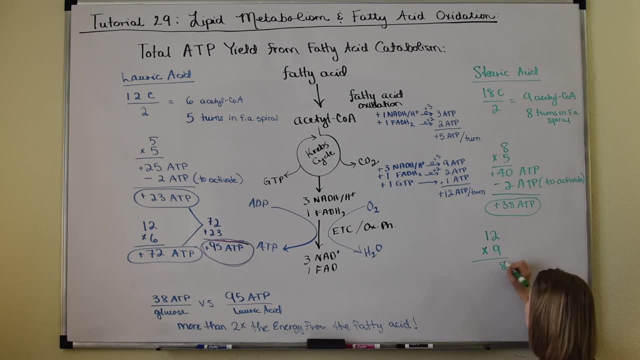 Turn, Or We Don't Just Have One Turn. We Have Nine Turns Because We Have Nine Acetyl Coenzyme To Break Down In The Spiral. 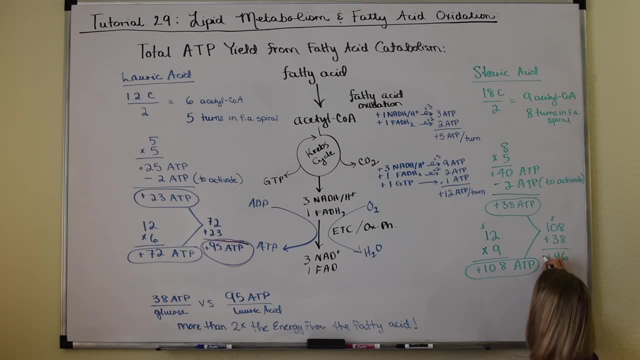 So We Got More Acetyl Coenzyme To Break Down. We Don't Have More Acetyl To Break Down. We Don't Have One More To. 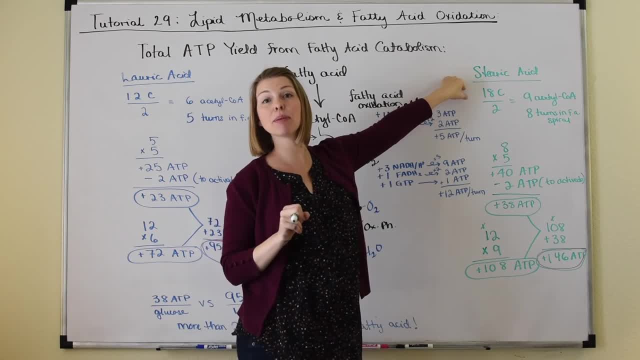 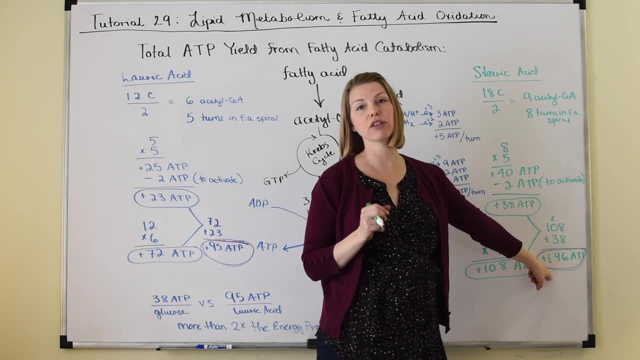 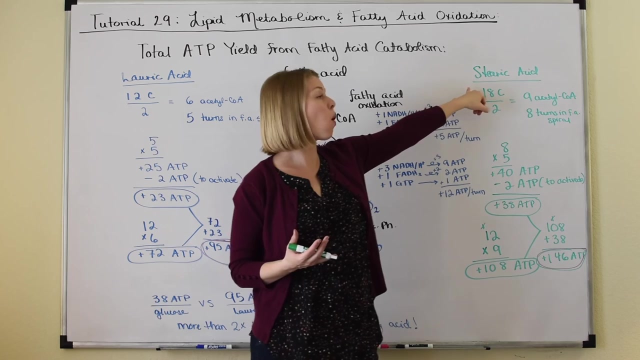 Break Down In One Molecule Of Steric Acid Being Completely Catabolized. We Get 146. ATP And Of Course, Remember That's The Max. 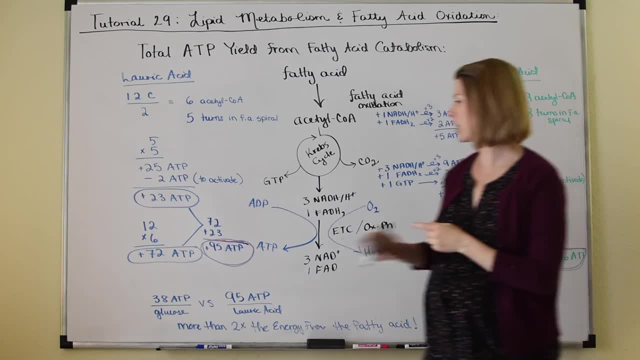 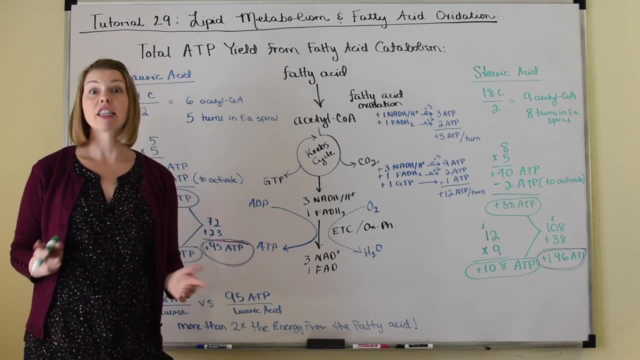 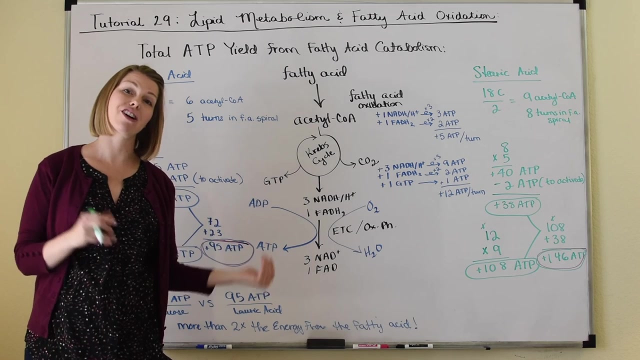 Yield, Because I Use The Numbers For Oxidation, Not So With Glucose. So When You're Calculating The ATP Yield For Glucose, Like We